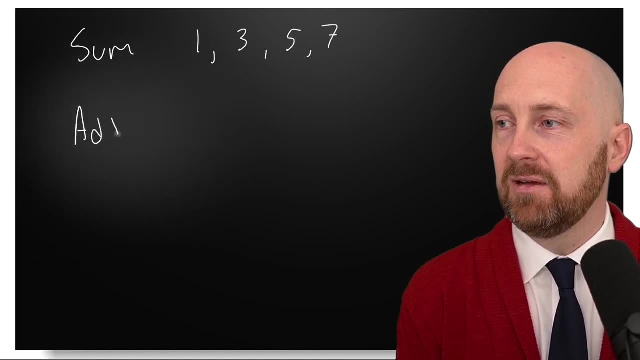 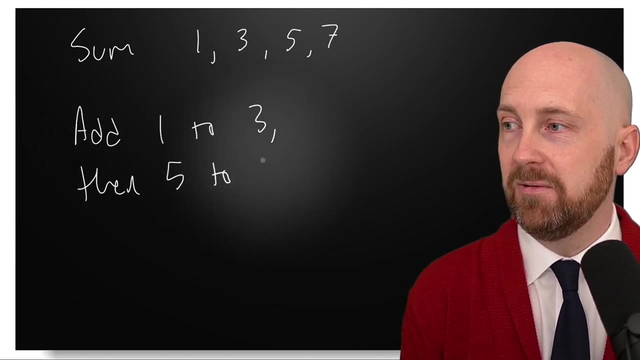 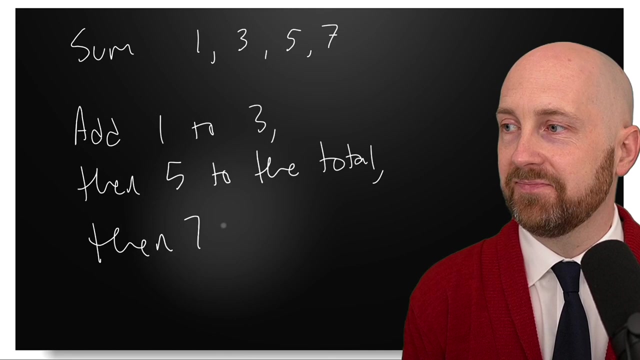 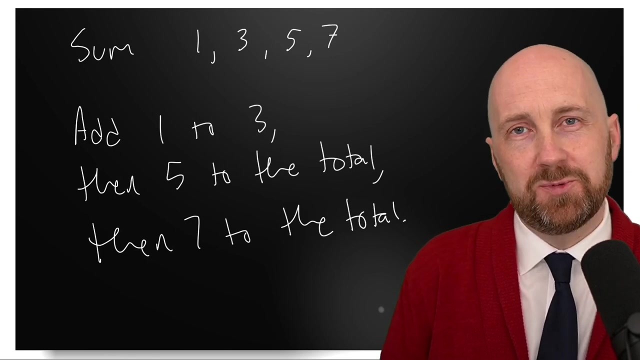 we could imagine, you know, add 1 to 3, then 5 to the total, then 7 to the total, right, And okay, well, we've been a little bit more specific here, but this is still. this is almost too specific, right. What happens when I? 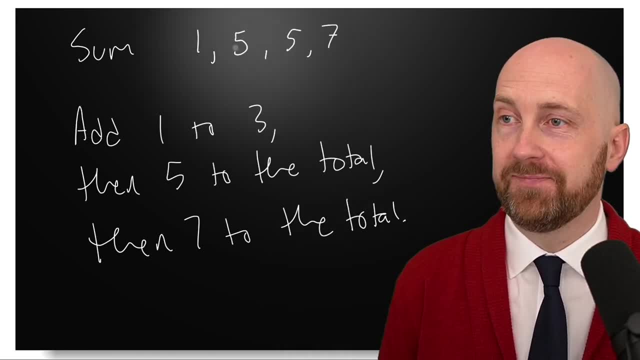 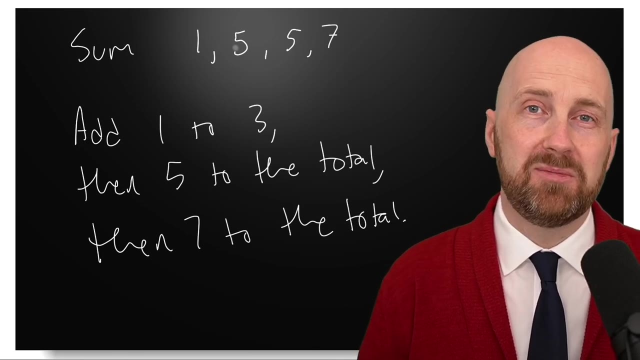 change one of these numbers to another, 5?? Well, what we just wrote, these instructions that we just wrote, are now wrong. right, So we've become more concrete and specific, but we have also- unintentionally, you know- fit the problem to too specific of a solution, right, Or too specific of a description of how to solve. 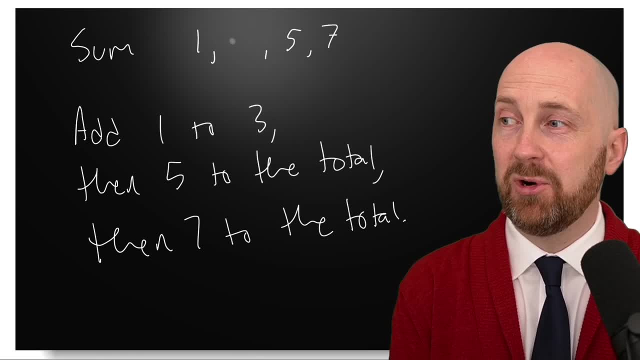 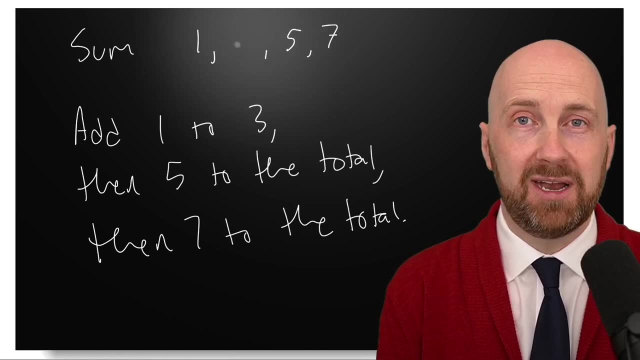 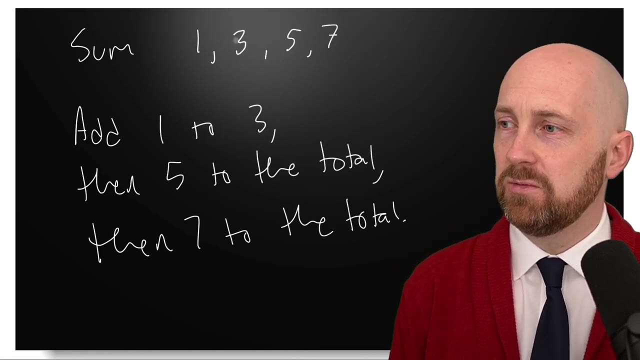 this, So our inputs shouldn't be specifically part of our algorithm. you know at their value level, right? So we shouldn't. when we think about how to describe an algorithm, we want to be a little bit more broadly, but still in a very precise way. So let's get some practice with 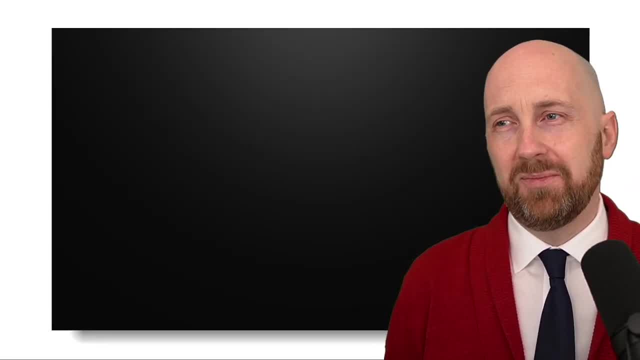 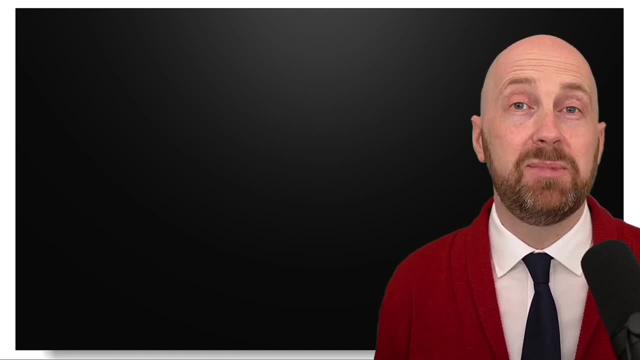 that, And what we're going to do next is think about: well, you know, we started from adding 1 and 3 together, but is that really the first step when you're trying to be able to add lists of arbitrary lengths? Well, let's imagine, okay, we've just been talking about summing 1, 3,. 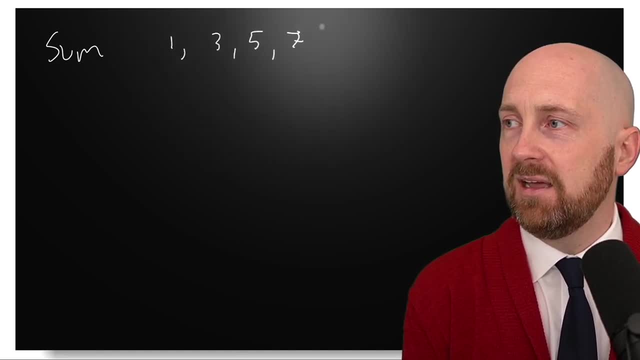 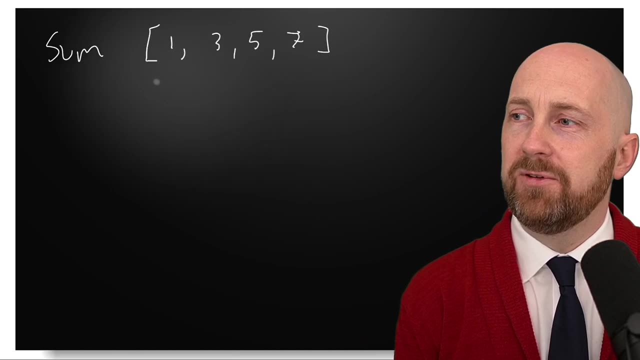 5, and 7 as our list, And let's imagine this is in Python syntax. So this is a list, literal here. Okay, that's fine. Well, what would be our first step if we were summing, you know, a list with just 1 in it? Well, we wouldn't add 1 to the next number because there 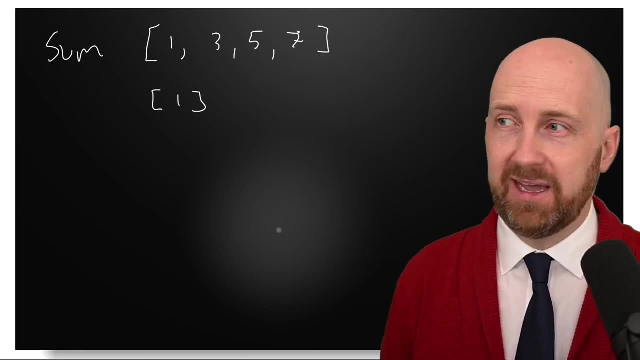 is no next number. So we're going to need to be a little bit more careful than that, And we're probably going to want to start from 0, right, Can you think of another reason why we might want to start from 0?? What's the sum of a list that has no elements in it? Well, 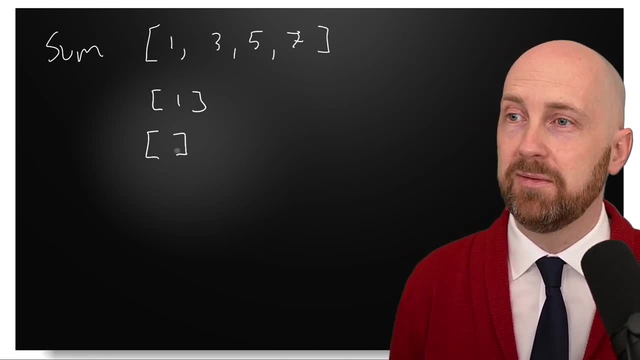 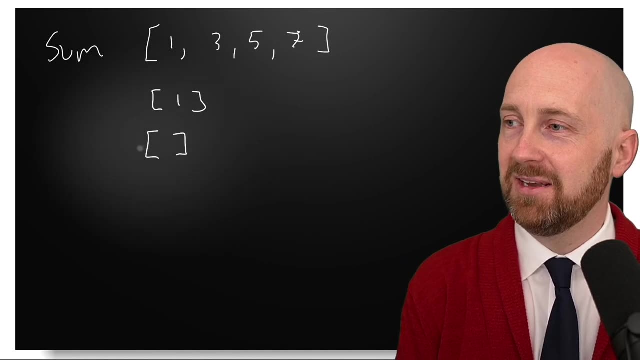 typically we would assume that that's the 0. It has no value to it. There's 0 elements in it. So when you add 0 elements up, you get nothing right. Nothing plus nothing is nothing. So let's keep track in terms of some total, starting from: 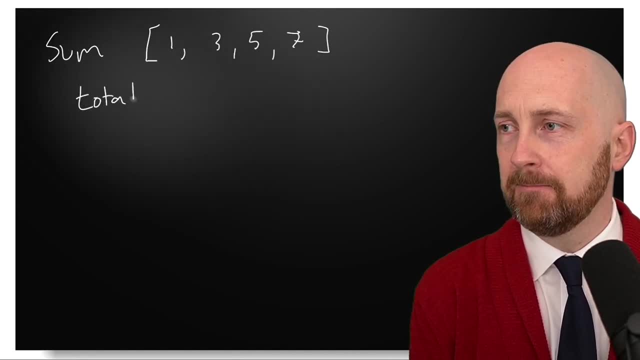 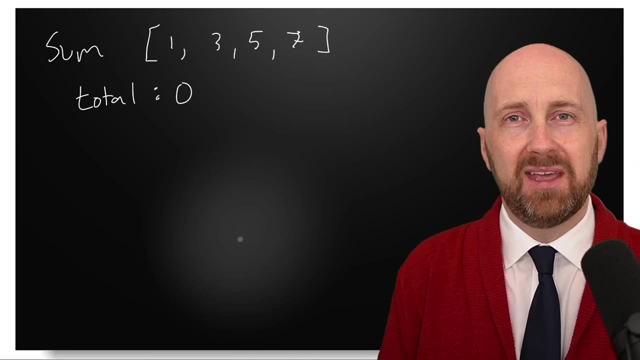 0. So we're going to have some total And it's initially 0. Now, previously we were thinking in terms of: okay, we'll add 1 and 3.. How can we be a little bit more generic than that and think: 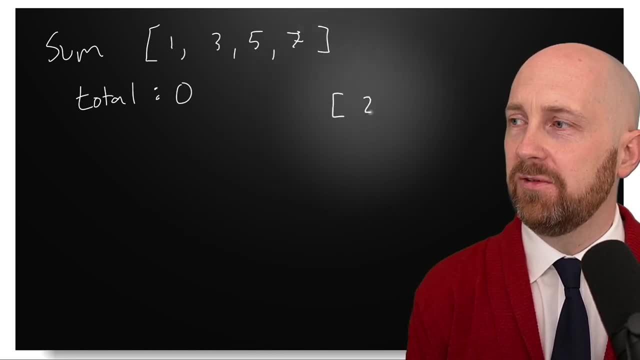 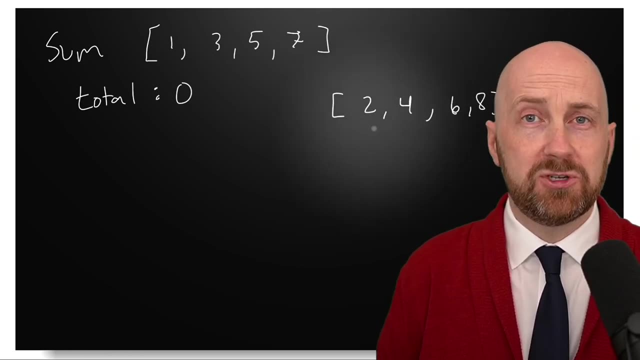 about, instead of 1 and 3,? well, what if our list was, you know, 4,, 6,, 8?? How could we think of the first two numbers, or the first, the very first number, more generically? Well, we want to think about adding items of a list as their particular place. 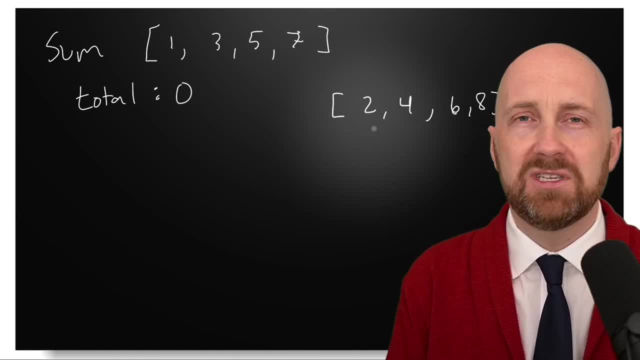 in the list, right? So maybe the first item in the list. What's the first item in our list In either of these cases? it's not necessarily the value 1 or 2. More generically, it's the item at. 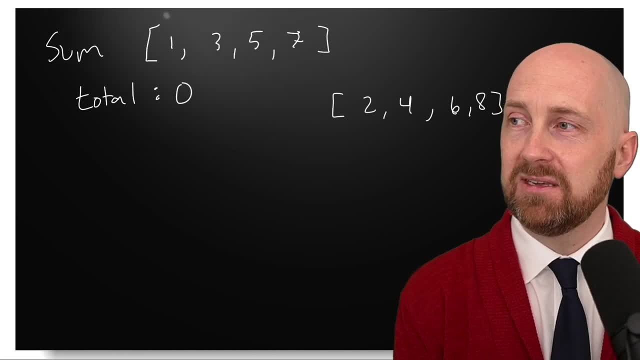 index 0,, right? So, remember, every list has a value of 0. So we're going to have to think about the first item in the list, its items or index 0,, 1,, 2,, 3, and so on, right? So if we imagine that, 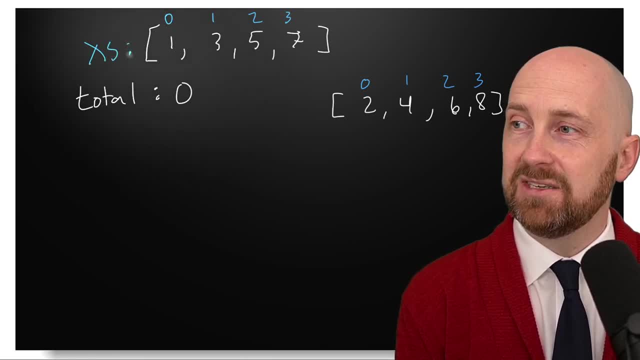 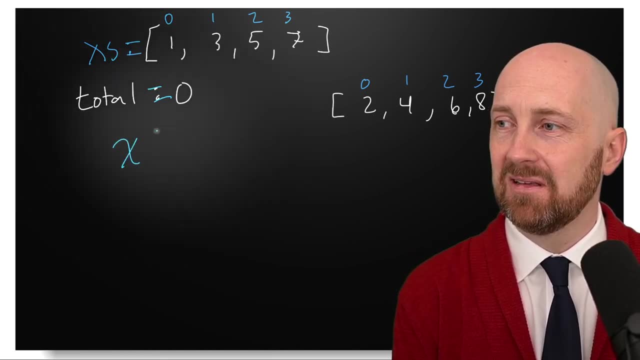 these are our. I'm going to just call this list x's. Imagine this is the list x's and our total is 0, right? So x's at index 0 would refer to the value 1 if we were, if x's was this list, But if 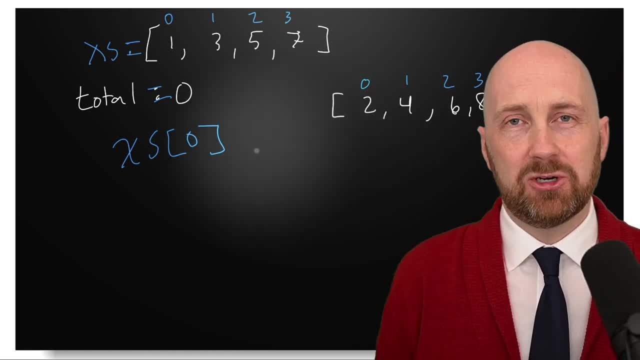 x's was this other list, it would refer to the value 2.. So by thinking in terms of you know a generic, you know our list, we're going to have to think about the value 2. So we're going to. 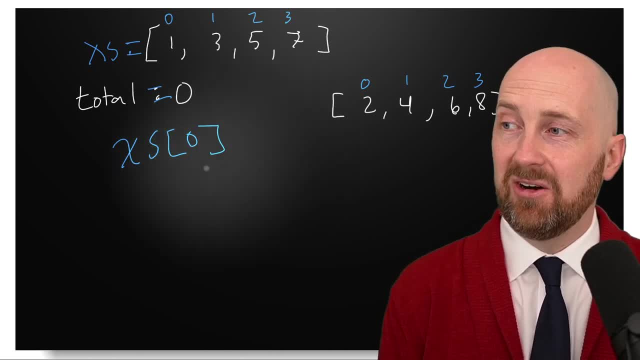 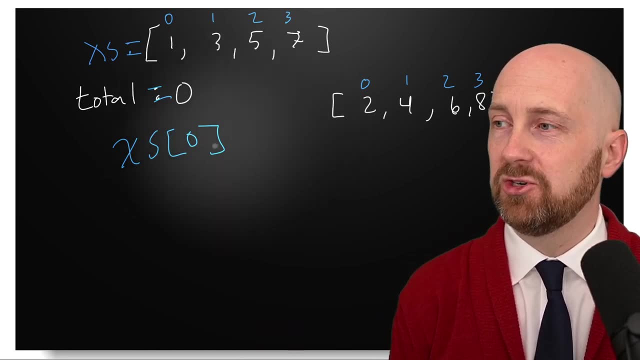 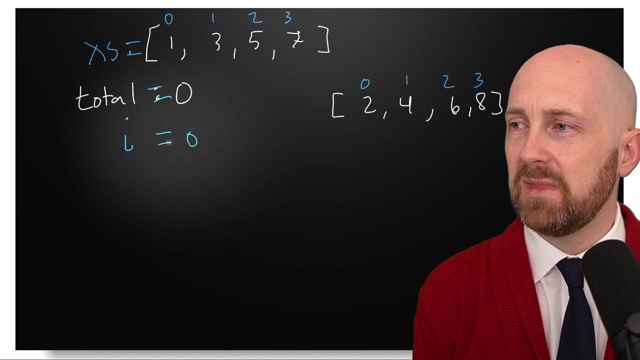 our list's name is, say, x's, And our index is something that we now need to keep track of, So index is going to refer to which item in the list we're trying to access and add up. So x's, let's think of this as index And I'll use the letter i to keep track of an index. Index is 0.. 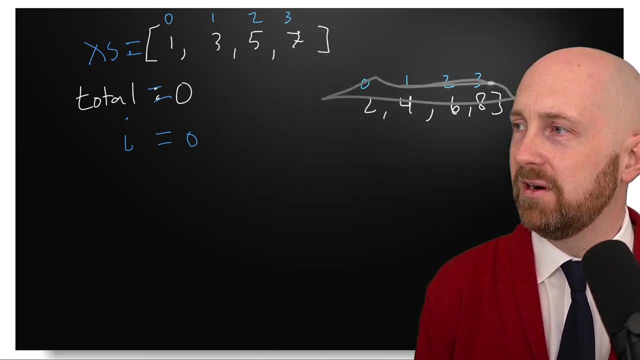 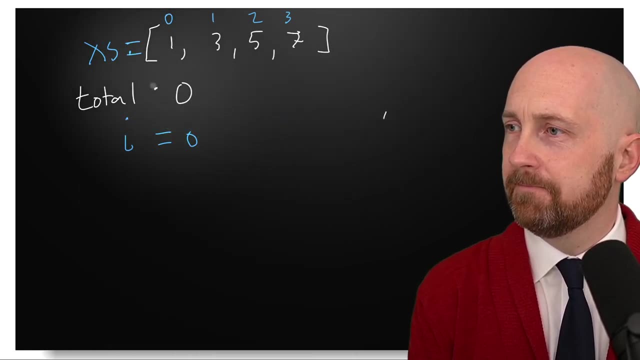 Now I'm going to, for now, just remove this other example here And we'll come back and talk about other examples in just a moment. All right, So how can we again still using English, but in terms of these two concepts- 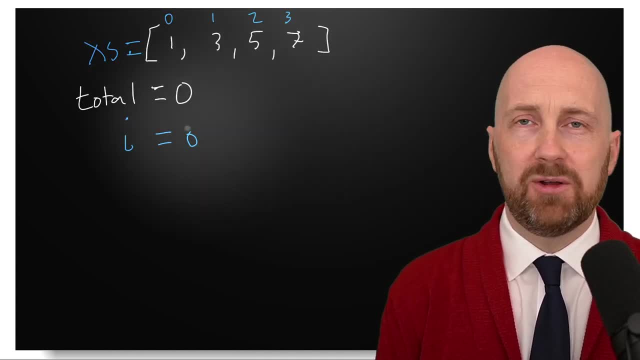 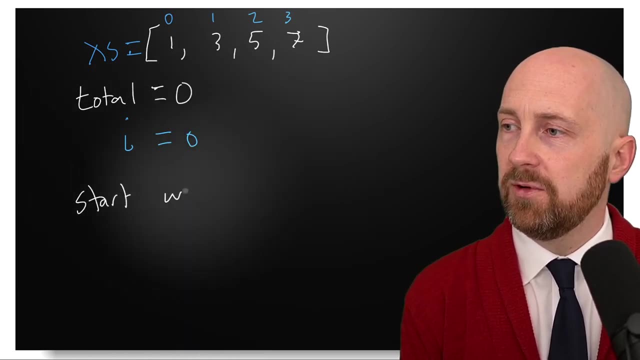 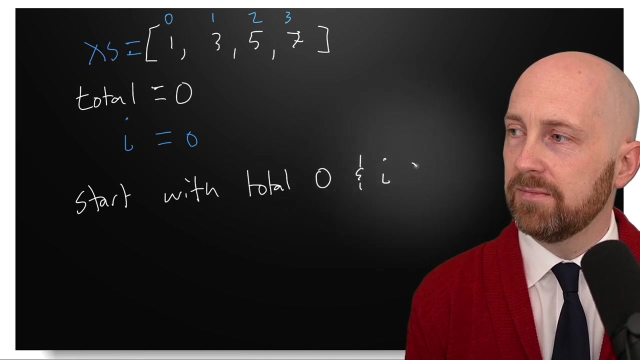 we now have an index and we have a total. How can we think of our steps a little bit more concretely? Well, we can start with total 0 and index 0, right, So that's step one. What's step two? 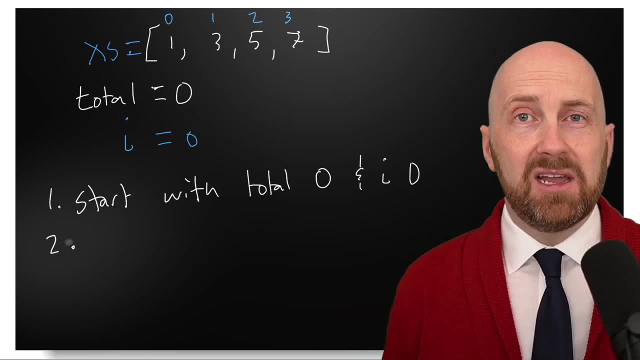 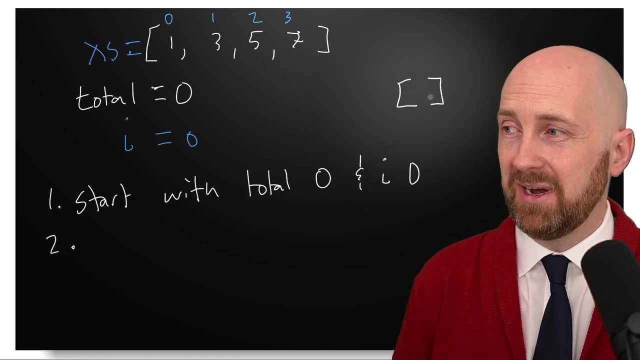 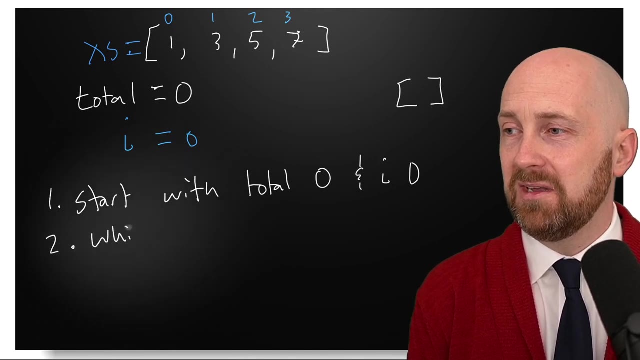 Well, before we go and add anything up, we need to know whether or not we're dealing with an empty list, right? Or whether or not the current index is still valid. Right now, the index is 0.. If we had an empty list, this would no longer be valid, So we want to just be sure you know, while the 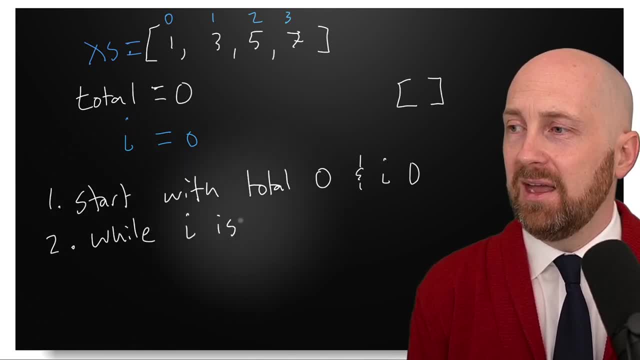 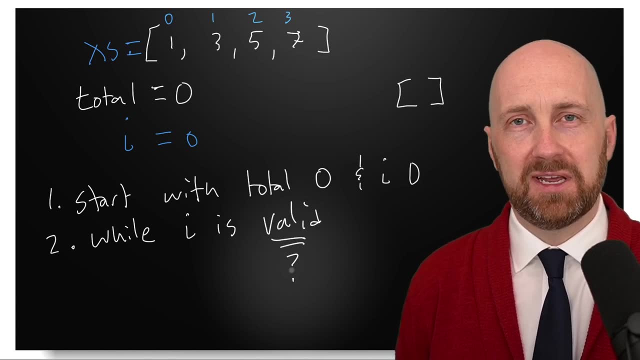 index is valid. But this idea of valid isn't very specific, It isn't very concrete. So what would it mean for us to have an empty list? Well, we need to know whether or not we're dealing with an empty list. What would it mean for i to be invalid? Well, if we're starting from 0, we want to be sure. 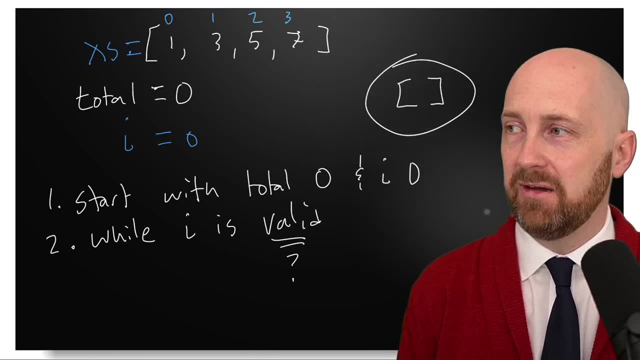 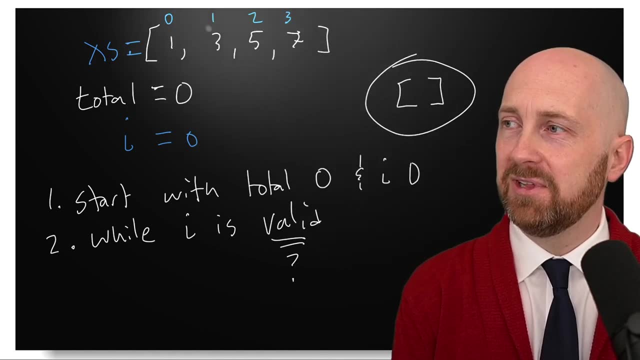 that it's. you know, i is less than the length of the list, right? So if the length of a list, in this case, is 0 and i is 0, then it's not valid. You know, if the length of a list is 4. 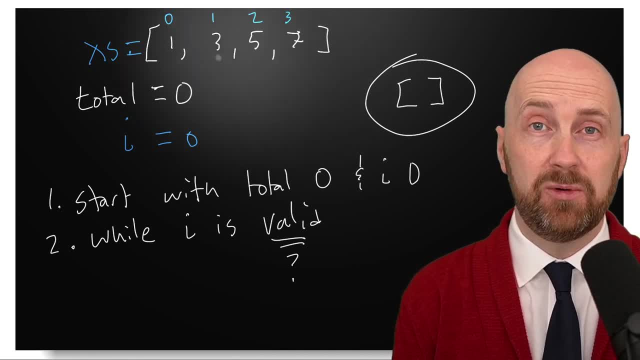 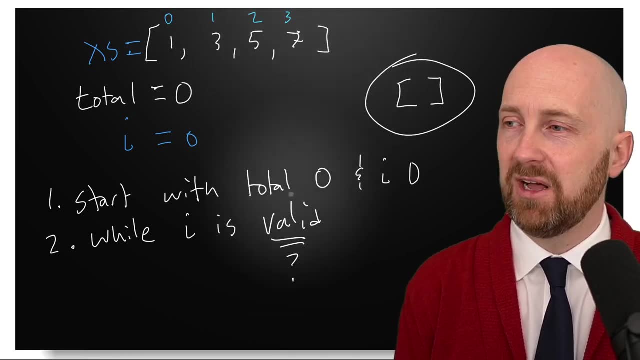 and i is 0,, 1,, 2, or 3,, then it would be valid. So any of those numbers are valid indices, But as soon as our index becomes 4, it would no longer be valid. So while i is valid, you know, maybe we'd. 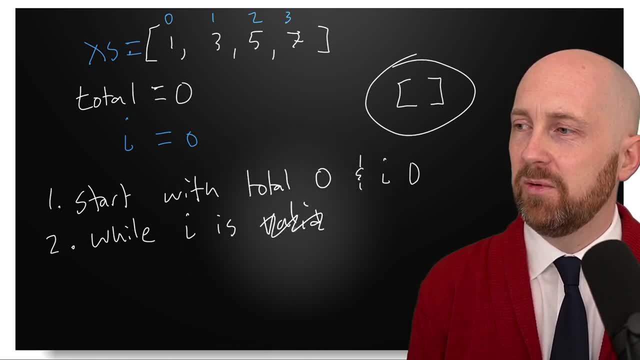 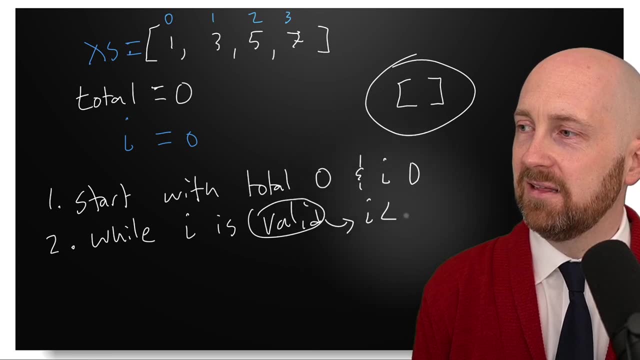 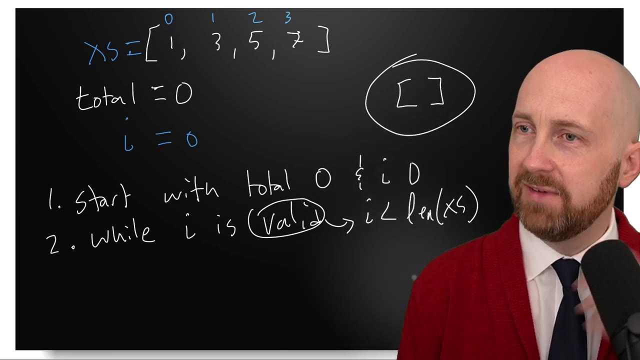 be more specific here And what we mean by that. actually, before, instead of crossing this out, why don't I just circle it and say: you know, i less than the length of x's, right, So i is less than the length of x's, which is what we mean by valid. And notice, we're kind of we're, you know. 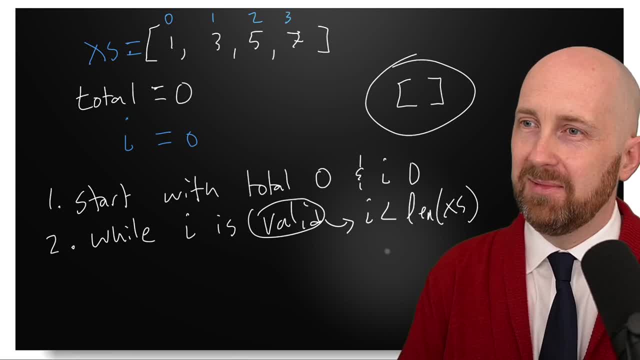 waving our hands a bit, just trying to feel out this problem and become more specific as we move through it. Okay, so if we, if we know that we have a valid index, that means that what we want to do is: you know. 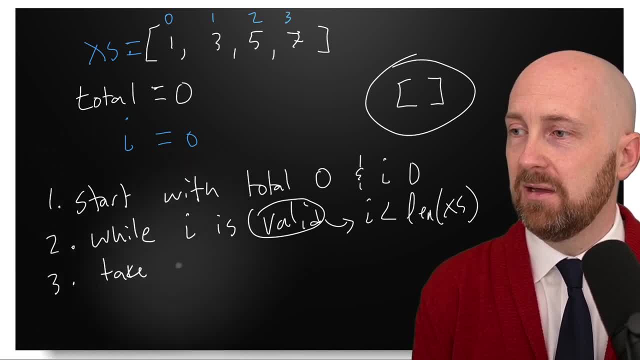 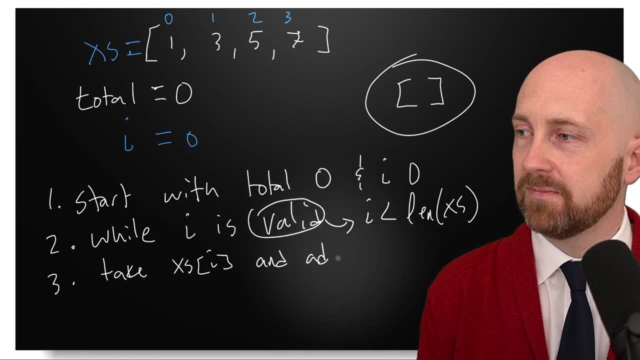 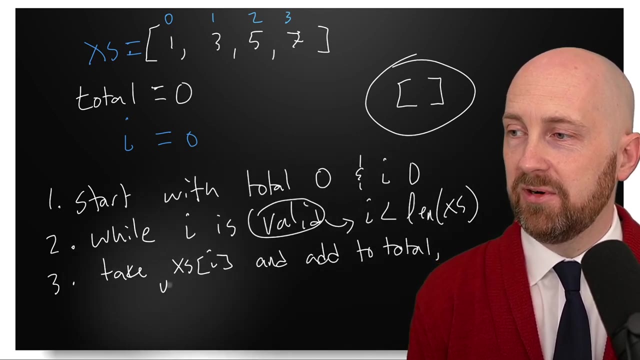 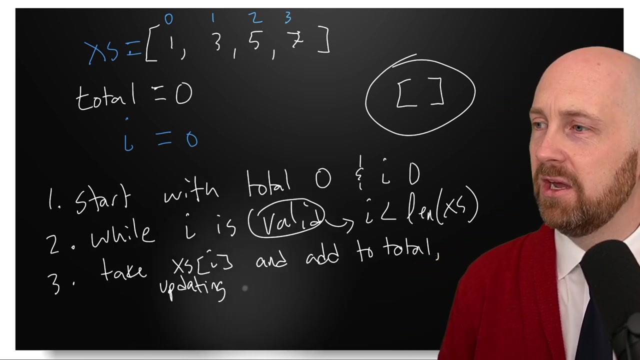 step three is take x's index i and add it to total Right Updating total, And that's important. We're continuously updating the total Each time we add a new item to it. Okay, So this will work for the very first item And this would be, you know. 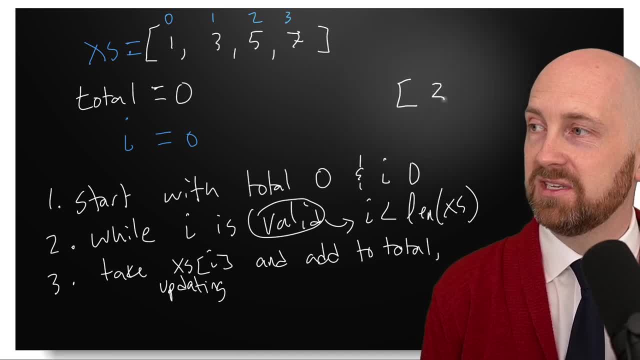 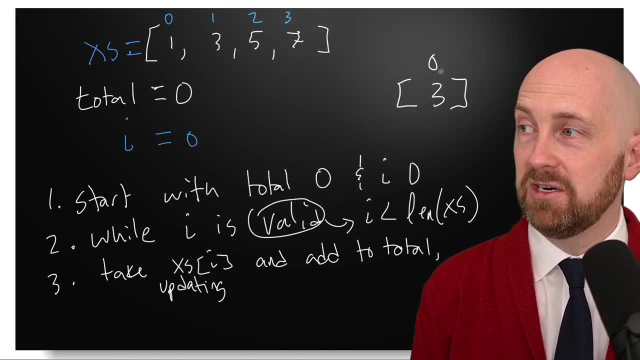 a good enough algorithm if we had. you know just what's the sum of the list with only three in it. Well, okay, well, i is zero There. zero is less than the length of this. the length of this is: 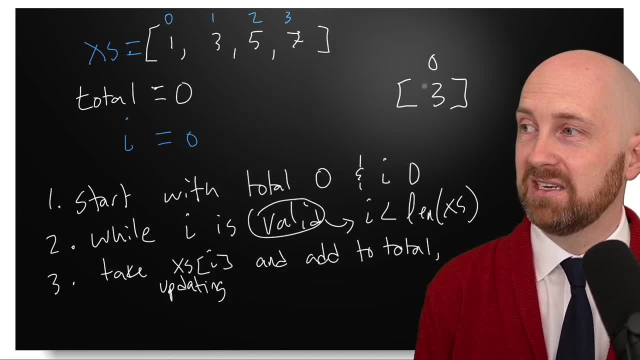 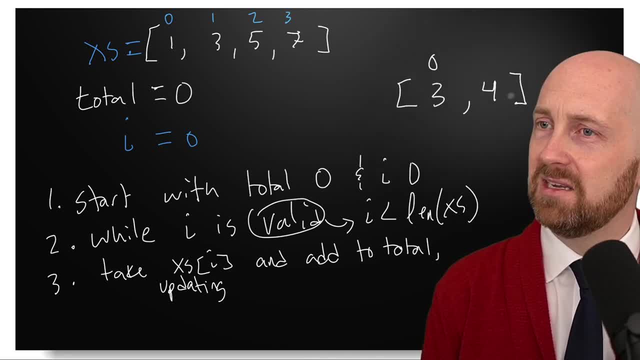 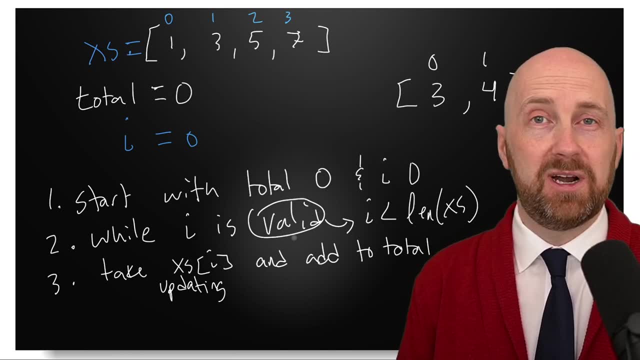 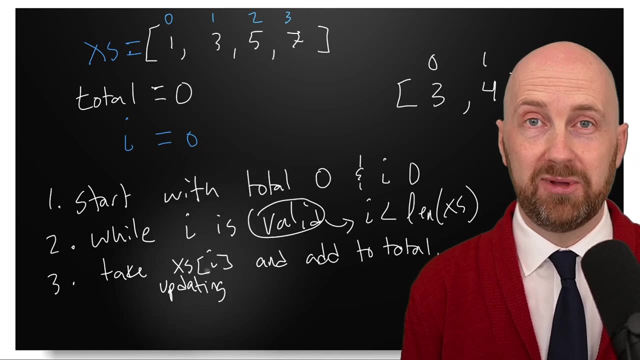 But you know this is no longer valid as soon as we have a second index right. So how do we make this algorithm handle the next index? And this is where the beauty of being able to index or subscript your lists and the ability to loop in an algorithm or a program really become powerful. 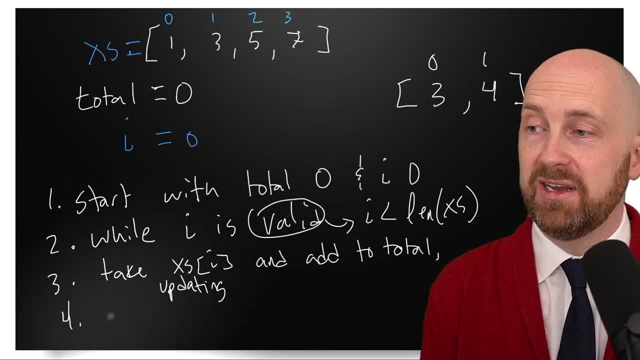 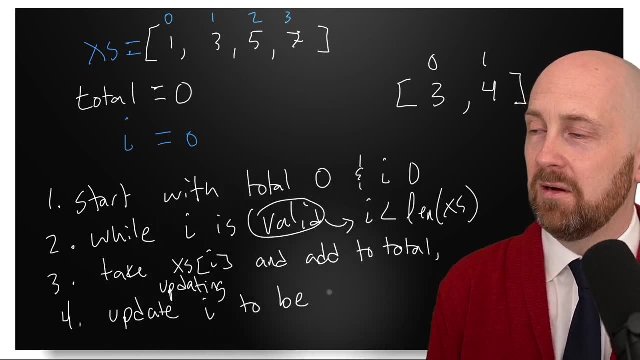 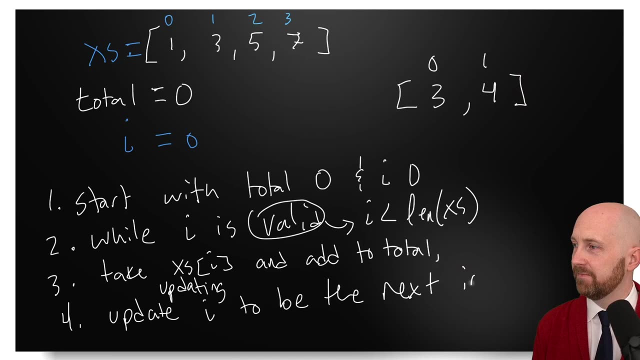 So what are we going to do? Well, let's update i to be the next index. So update i to be the next index. And what do we mean by the next index? Well, you know, if we're trying to be a little bit more specific about this, 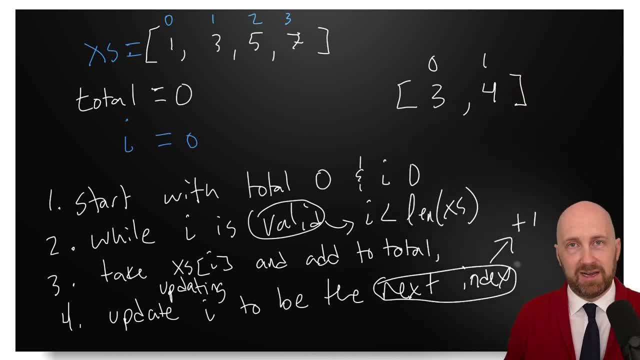 you know, this is the same as you know, plus one, right. So if i is initially zero, the next index is one, the next index is two. So we're going to increment i by one, So that English can be a little bit. 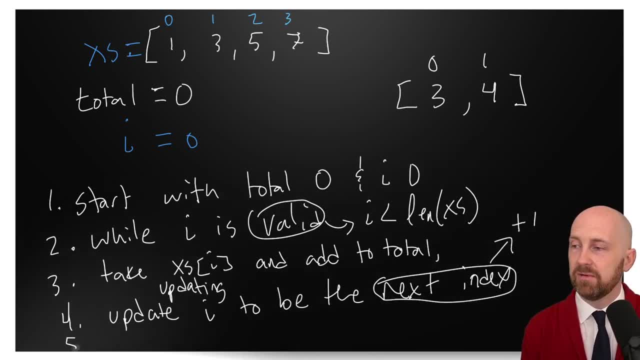 And after we've done that, what do we do? Well, this is where the looping comes into play. We're going to go to step two, right? So this is the end of our loop, And we're going to go back to step two. 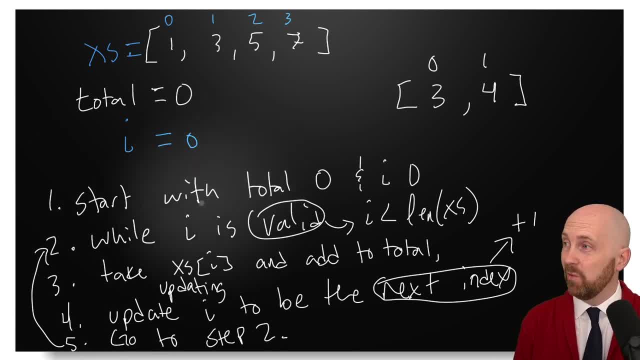 And we're going to ask again: okay, well, we just changed i. i is now one. If we were thinking about this simple example we would access, we'd ask: is that still valid? So one is less than the length of this, which is two. 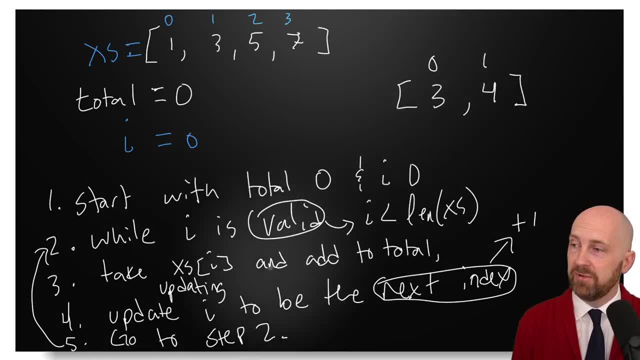 So, okay, that's still true. Then we're going to go to step three, which is, take the next item i at index one, add it to our total. Now, total in this case would be seven, and continue on. And if we were to think about this in terms of, you know, 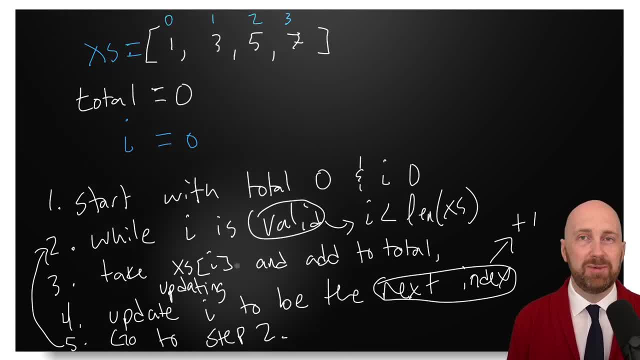 our original example with four elements in it. this same algorithm should hold right. We should just be able to move on to the next index. take its value using the current, you know, x's at index i. So index one would be three, index two would be five, index three would be seven. 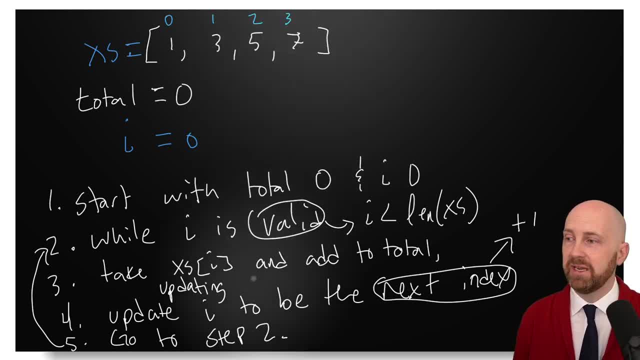 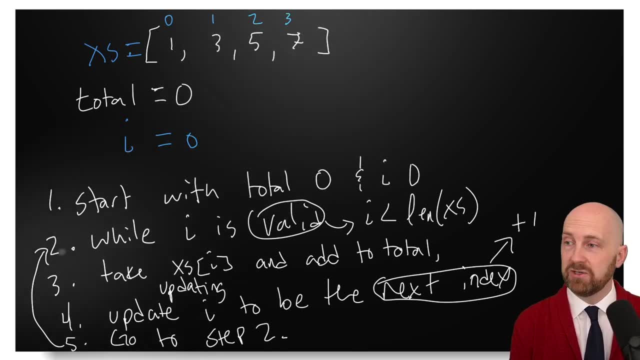 Each time we do that, we're going to be able to move on to the next index. We update our total to add this amount to it, And then we update our index to go on to the next index until we reach the point at which the index is no longer valid. 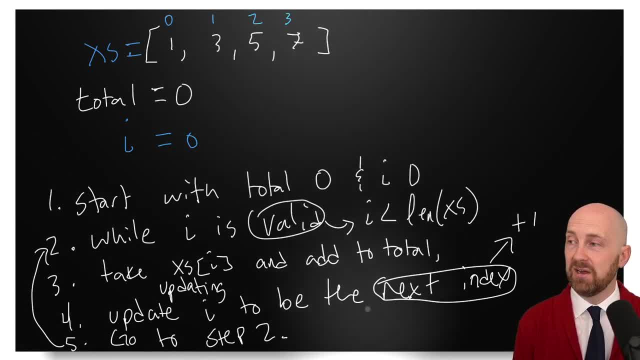 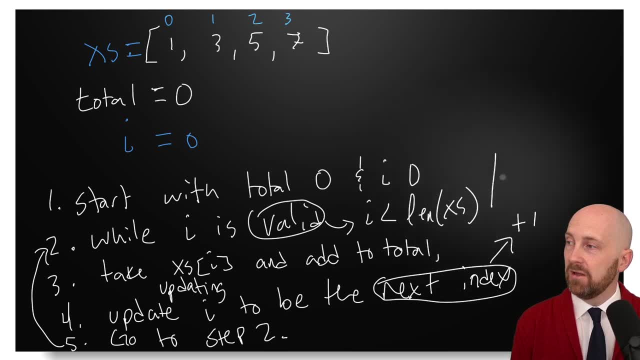 So when step two becomes false, we need to do something else. So when i is valid, we're going to do, we're going to go into step three, Otherwise we're going to- and this is going to be kind of sloppy here. 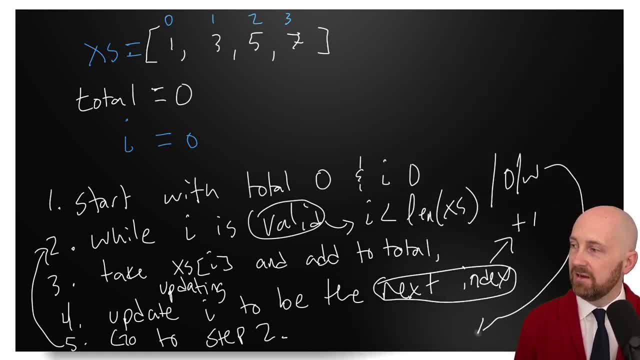 but otherwise, if i is not valid, you know we're result is total, right? So whatever is left in our total variable after we've moved through this algorithm is going to be the sum. okay, So this is sort of some intuition behind how you're going to sum a list of numbers. 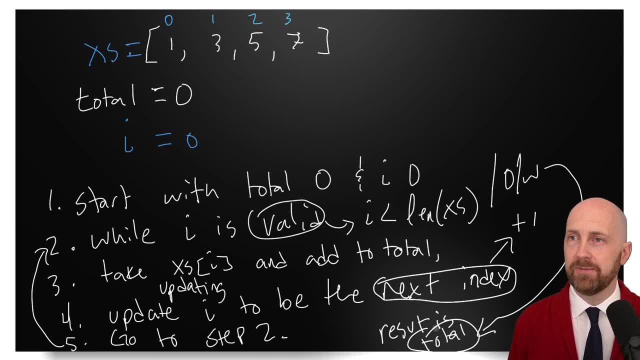 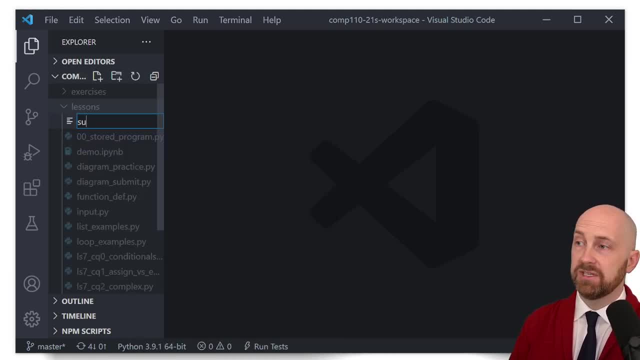 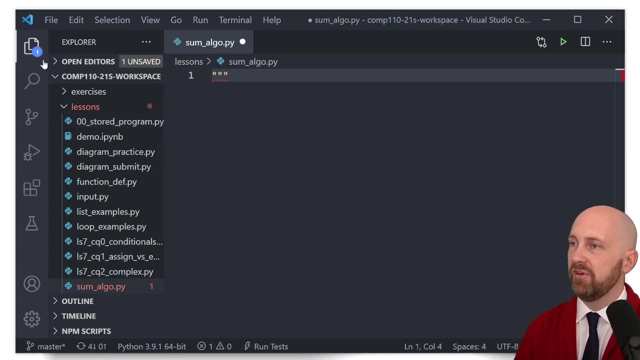 Let's jump into actual VS Code and carry this out right. So I'm going to set up a file that will be named. let's call it sum. I'll go dot pi, right, And let's just add a description here, that is, examples of lists and loops. 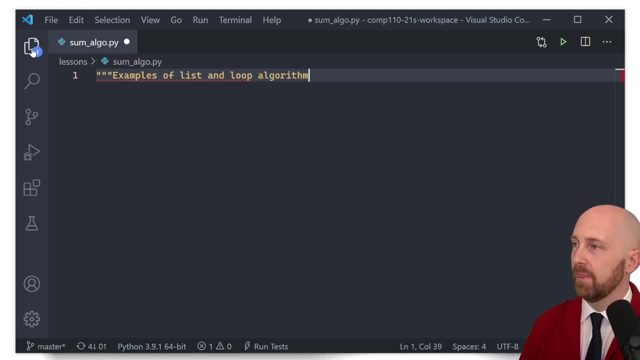 list and loop algorithm. okay, Let's say we wanted to define a function that could carry out our summation, right? So define sum algo, right? So what was the input to our summation? Well, it was: we wanted to have a function that could do a lot of things, right? 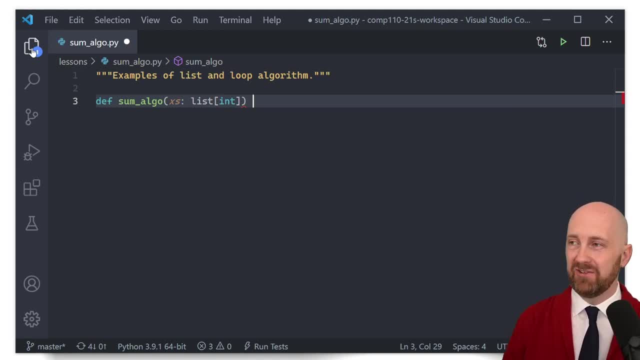 So we're going to run the function right And we're going to name it XS, right. So XS is a common shorthand name for just an arbitrary list of of of calling numbers, And the result of this algorithm is an integer right. 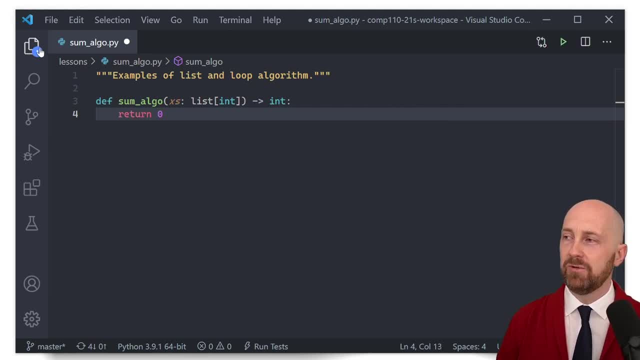 So for now, I'm going to make this what we call a skeleton of a function, and it's going to have all the components to make it valid, but it's not going to yet be a valid function, So let's add a docstring here. 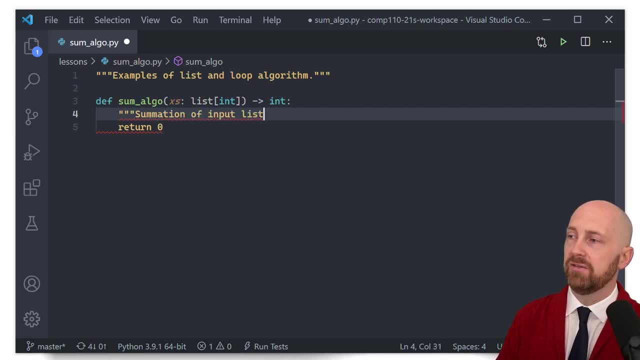 summation of input list is returned right, great. and you know this is a. this function isn't correct yet, so how do we go from having an incorrect? but it does return the correct type, right? so this return statement: if we were to call some algo from somewhere else in our program, it would return zero. 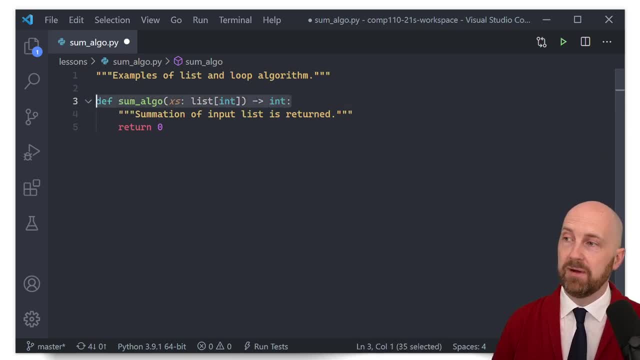 that actually satisfies the, the return type of our function definition. so this is a valid function. that's incorrect, and you'll commonly come across those, and that's usually your best starting point when you're trying to implement a function like this. okay, so we've got x's and let's go return. 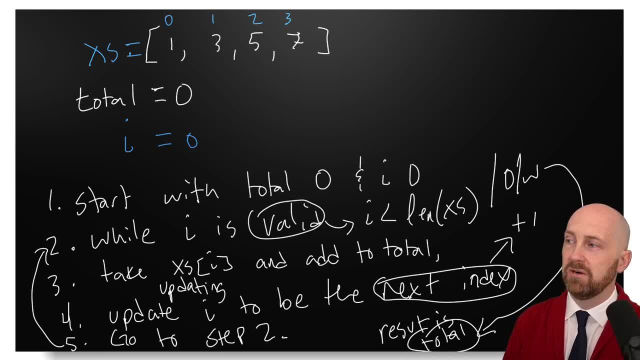 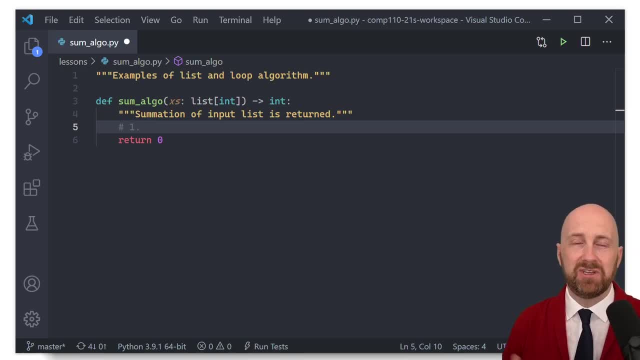 back to our notes. so our notes were start with a total of zero and i of zero. so what i like to do is take my steps that i've written out in english, sort of the overarching goal of some task i'm going to carry out in code and reproduce those as comments. first, 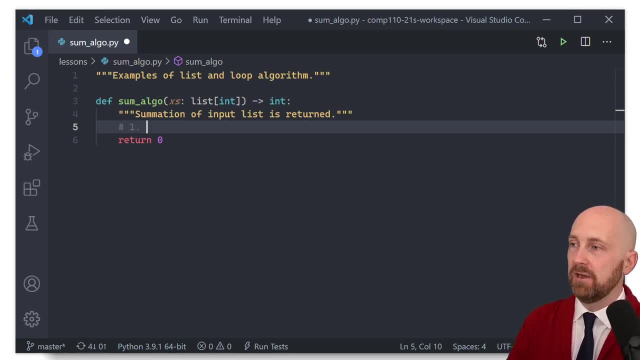 So I'm going to add a comment here. So step one was: initialize total and index i to zero, right? And before I even worry about implementing this as code, I might go ahead and jot down some of the other steps, right? So that was step one. 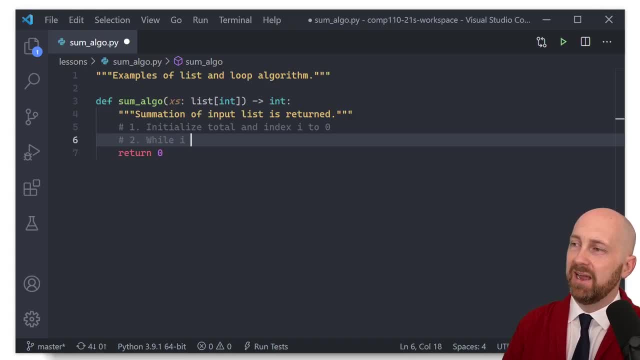 Step two: while index i is valid, meaning i is less than length of our x's list, right? And I'm going to indent to say: you know, okay, when two is true, right? Then what do we do? Well, we said we're going to take x's at index i and add to total. 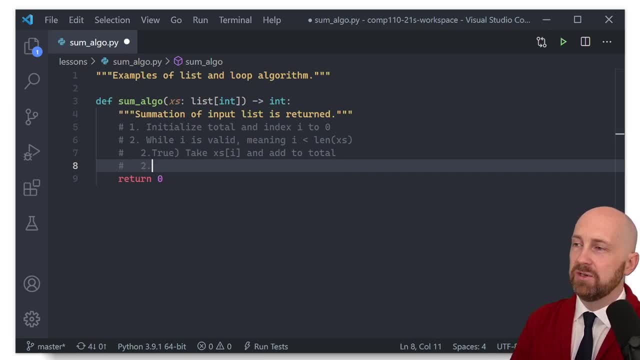 Right, But that wasn't all we wanted to do when two is true. So the next thing we would do inside of this what's going to become a loop, is we need to be sure that we move our index to the next index. 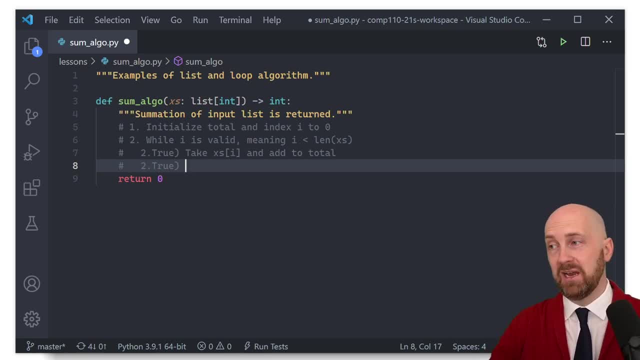 So we started from index zero, the first item in our list, and now we need to move on to the next index. So increase i by one, moving it to the next index. Okay, Now there was this. also there was a case where two is false right. 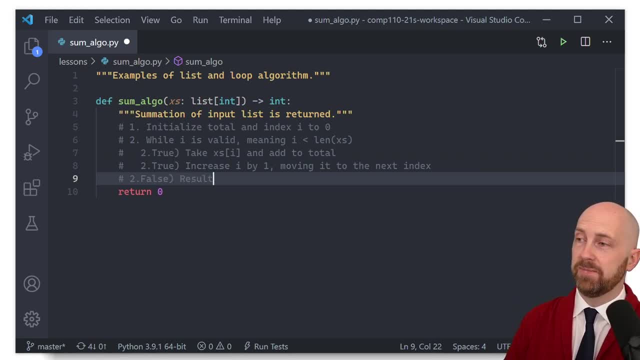 When two is false, the result is stored in our total variable right. This is sort of where we're keeping track of the accumulated result. At each time we sum a new number to our total, it's being stored in our total variable. 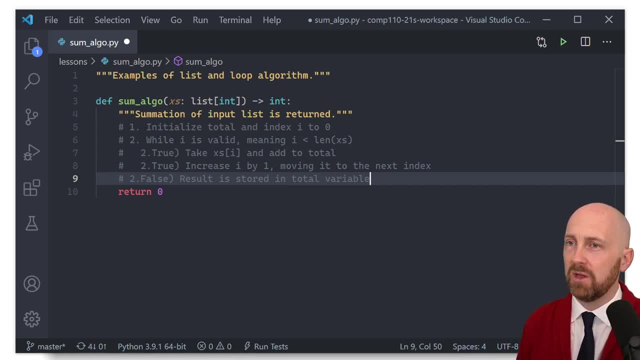 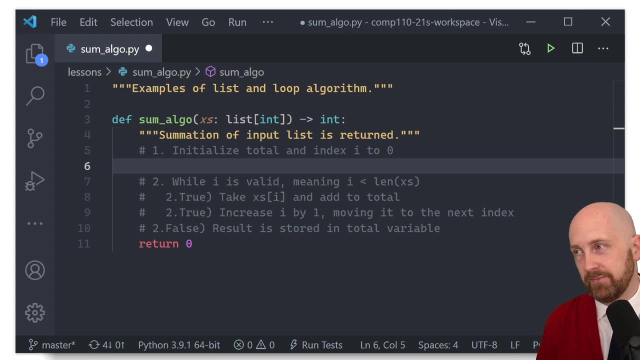 And ultimately, that's going to be our result. Okay, Now that we have these steps in English, let's try turning them into code. Okay, Initialize total in index i to zero. So total Is going to be an integer variable and initially zero. 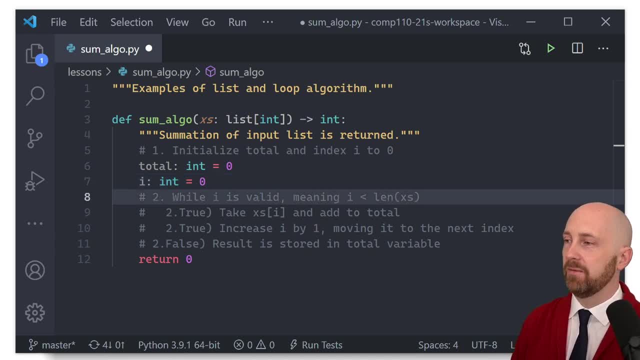 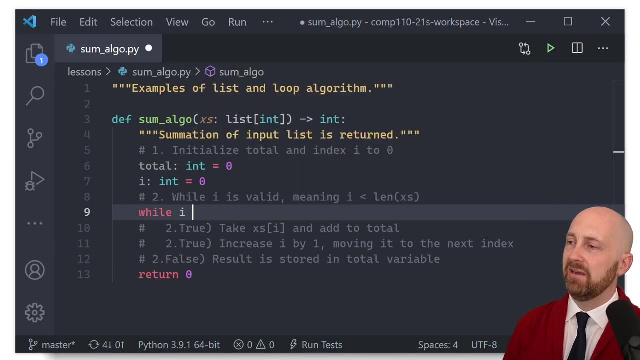 i is also going to be an integer variable and also initially zero. Okay. While i is valid, meaning i is less than the length of x's- Okay. So while i is less than the length of x's, Okay. Now that intuition is sort of nuanced. 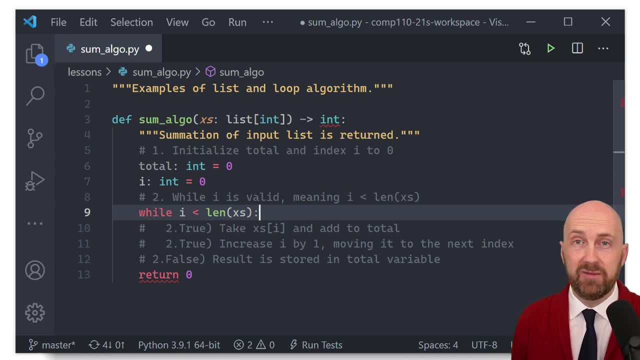 but we previously talked about. if you want a loop to run a specific number of times and you start, you're going to have a loop to run a specific number of times. So if we run your counter variable, which is i or index, here at zero, 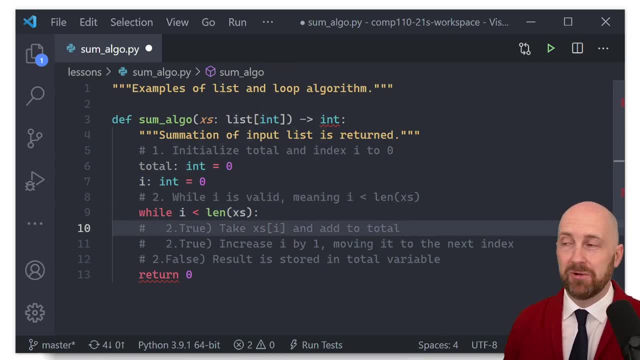 then we want to loop, while that counter variable is less than the total number of iterations. we want to run because we're counting from zero. There's this off by one factor where we have to shift everything by one, And because our length, the length of a list. 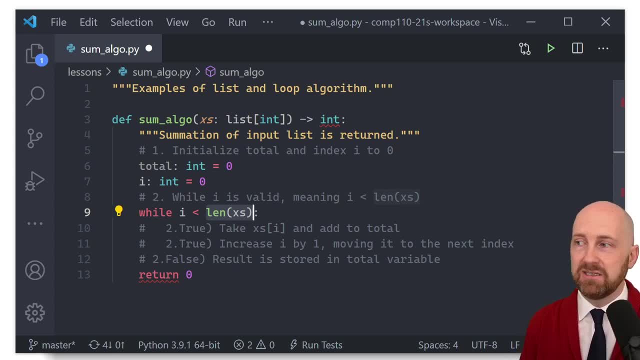 If we have one element in our list, the length is one in the first, index is zero, And so that's what's going on here. Now, the next thing we want to do is actually be sure that these, the next two steps. 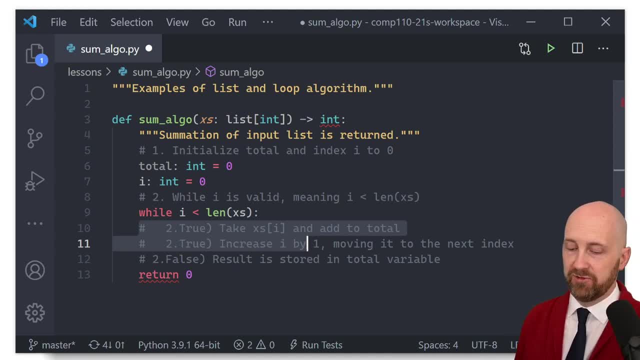 are contained inside of the body of this while loop. so one of the things that we haven't discussed yet is: you know, if you want to indent a number of lines of code at the same time, how would you do that? well, you know one way is you know, you select the beginning of each line and you tab. 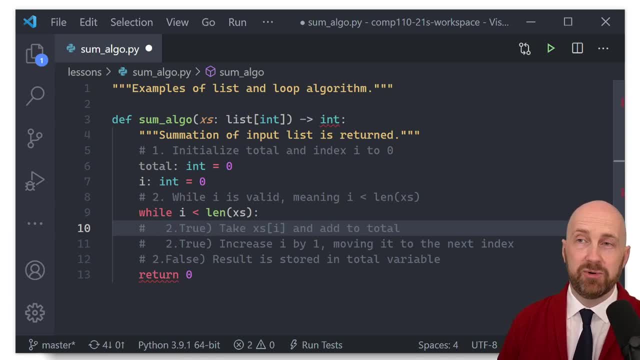 them in individually, but this is such a common operation when you're programming that what you'll tend to want to do is select all of the lines that you care about. so i'm going to use my mouse to select both of these lines, and you don't have to select the whole lines as long as you have parts. 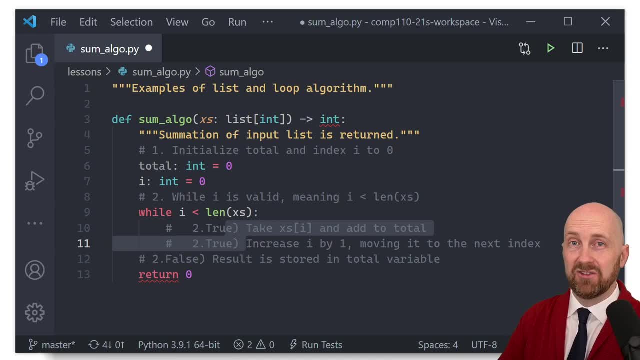 of the line selected and then if you press tab it's going to indent every line you have selected by one. and then if you hold down your shift button and press tab again, the shift will sort of do the same thing in the opposite direction. i like to say unindent, but i don't think that's actually. 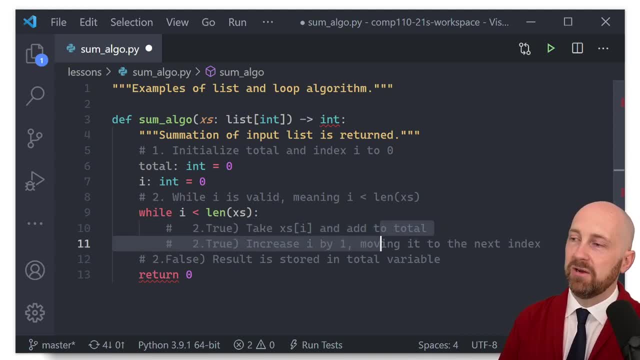 a real word, okay. so, uh, you can very quickly, you know, indent unindent. i'm going to indent my uh directions here and say, okay, well, what do we want to do here? we want to take x's and add it to the total. that means we're trying to reassign at total. so this is one of the things that we need. 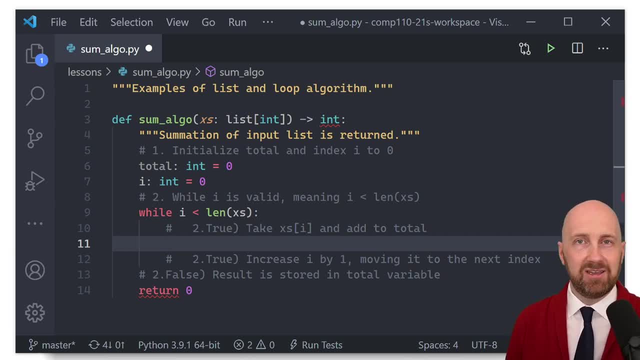 of those cases where, when you're turning english into code, you have to be comfortable with: well, what are the statements that are valid programming statements? so we know a statement like total is assigned. total plus x is of index i. but we just learned that we can actually write this with a. 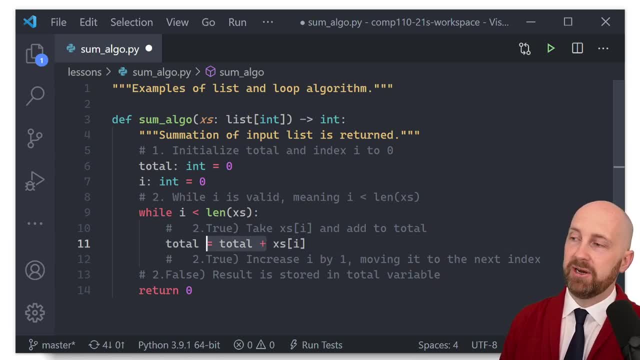 little bit of shorthand using our relative reassignment operator. so this is the same as saying: total is incremented or increased by the value sort of x is index i. again, the first time this loop runs i is going to be zero. so we're saying what is give us the take the current value. 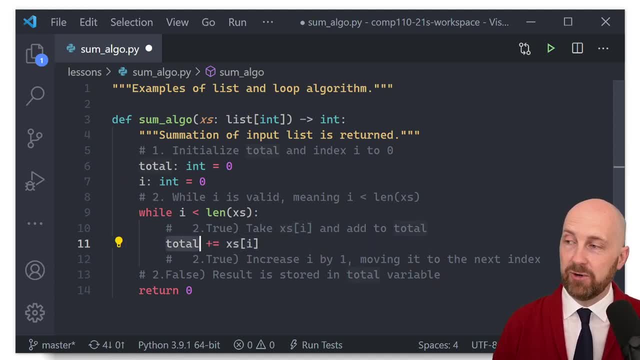 of the, the first item in our list, and add it to our total. but as this is written, we currently have an infinite loop. right, we're not changing anything about nothing in this loop is changing anything about this condition? we need this condition to ultimately become false at some point. 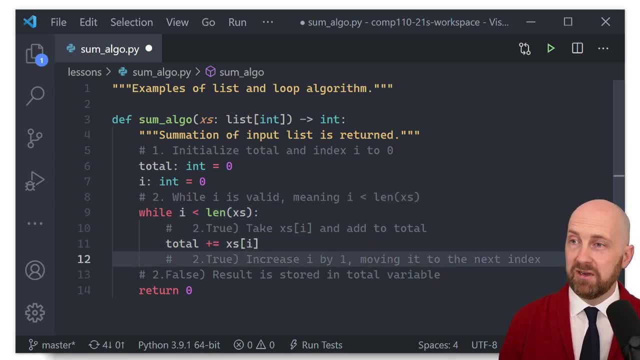 in order for this not to be an infinite loop. so, more logically, what we want to do is: we're going to have an infinite loop, so we're going to have an infinite loop, so we're going to is be sure that we move our index to the next index. we started from index 0, we added the first. 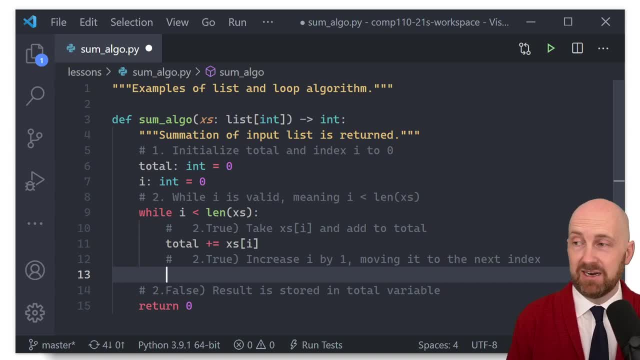 element of our list to our total. now we want to move to the next index. so how do we do that? well, we could say: i is assigned i plus 1. or, as we just learned, i plus equal 1 increases i by 1.. great notice that this means each time this loop iterates. 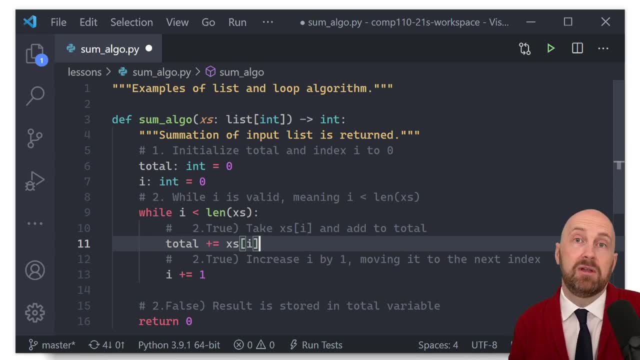 we take the value stored at the current index, we add it to our total and then we move to the next index. we take that index, we add it- whatever item is stored in that index- to our total, we increment our index and we keep following out this procedure or this process. 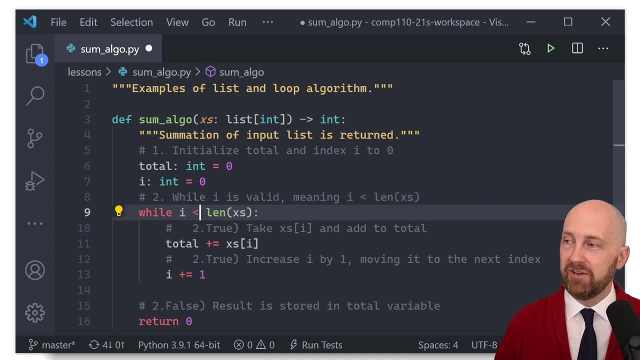 until this is no longer true, right, so once i once the index we're looking at is no longer a valid index, meaning you know, there just isn't an item stored there in our list. we've got an index that's beyond the end of our list. that's when we're we're done with this loop. we're. 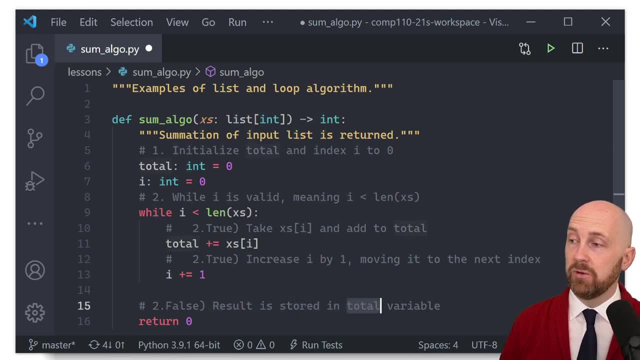 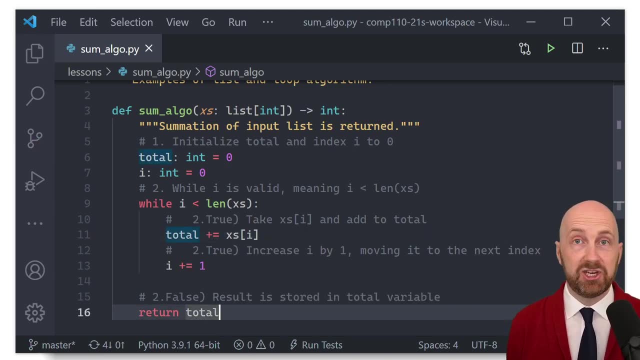 going to move on to the next one, and we're ready to return our total. so our result is stored in our total variable. so that's probably what this function should return: return total. great, all right. well, now we've written a generic algorithm. let's actually see if this works. let's try testing. 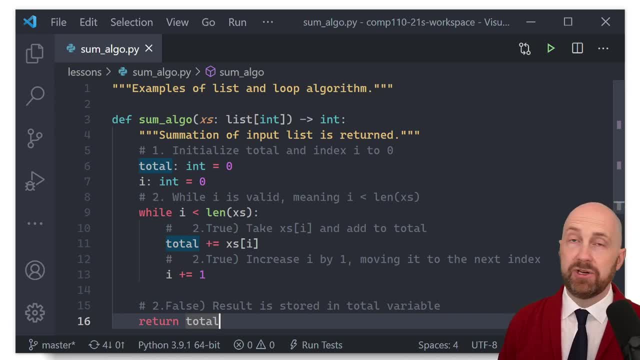 this out. um, one of the things i want to show you: uh, when you're writing a program or a function like this and we're abstracting away this process, this, this function, is an abstraction of the function. we don't have to think about all these details in a very low level like we just did. 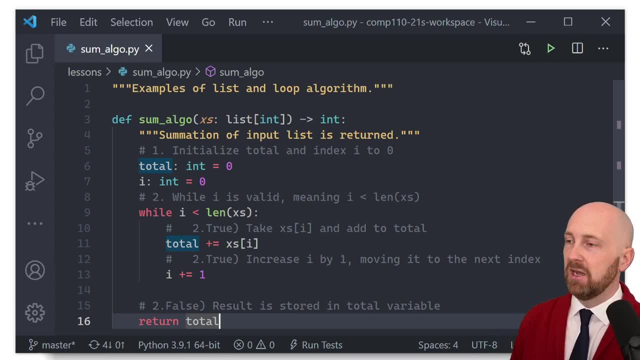 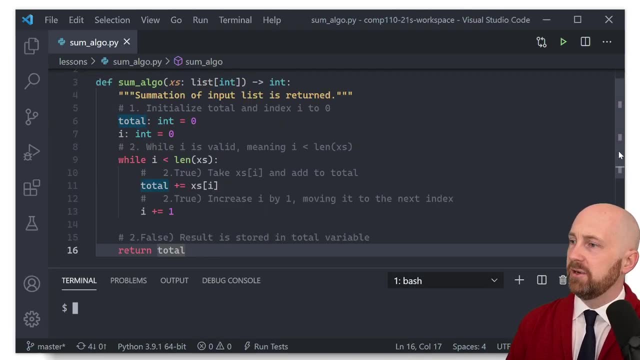 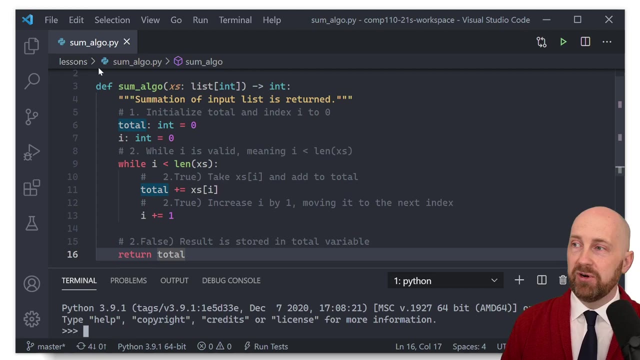 we can think, hey, i want to add up some numbers, so i'm going to use my sum function. so how can we actually use this in a vs code, repl? let me make this a little bit smaller so it all fits. what i'm going to do is i'm going to start up a repl and now i'm going to import this function. 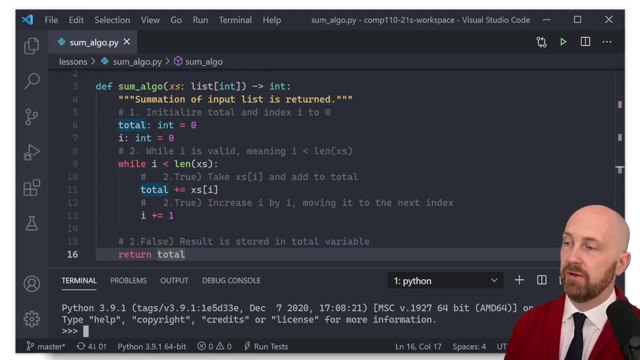 right. so this is something new in in our course. i'm going to say: from lessonssum algo, import some algo, right? so this is a little bit funny, because i named the file here sum algopi, lessons and then the module name is some algopi, and then we also named our function some algopi. 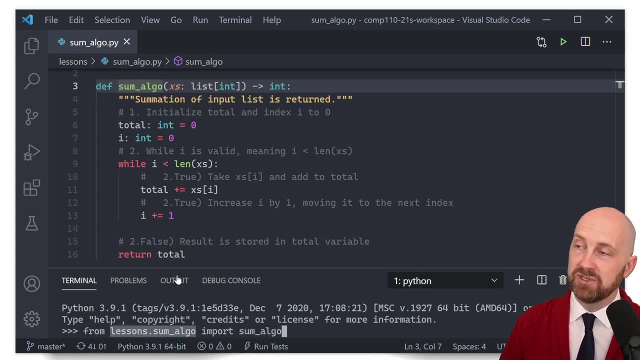 so that's why we're saying this is saying from the package lessons, the module, some algo, which is this whole file from the module residents, from lessons to the modulerésonsumargopy- going to import this function. if we had more than one function here, functions had different names. 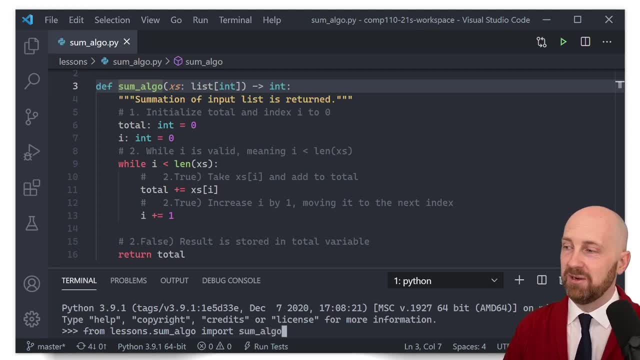 we would have said: import, you know, function foo, if there was a function named foo. okay, so i've imported the sum and now let's try, you know um, seeing if it works. so, sum algo, and then we're going to give it, let's say, a list literal of the empty list. let's start with something simple. 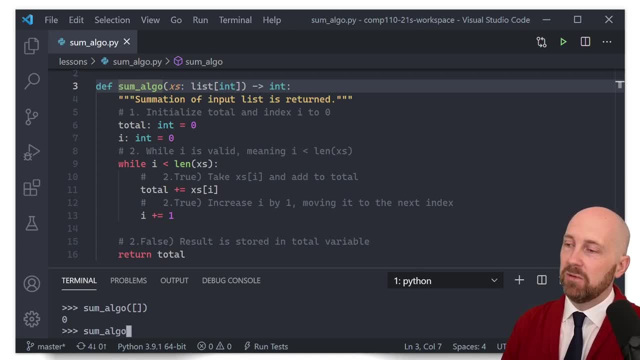 boom, the sum of the empty list is zero. that's great. well, what about the initial item, or the initial list? we started with one, three, five and seven and we calculated that, as humans, to be 16, and, wow, it looks like. uh, our, our implementation here is is letting us know we're we're correct. 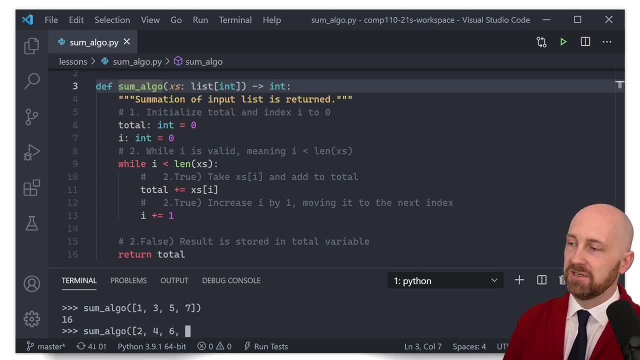 we could also try some algo of say two, four, six and eight, just to convince ourselves this is a generic algorithm that works for, uh, different numbers. and boom, what do you know? we've got uh, 20. two plus four is six. six plus six is twelve. twelve plus eight is twenty. great, uh, some algo. 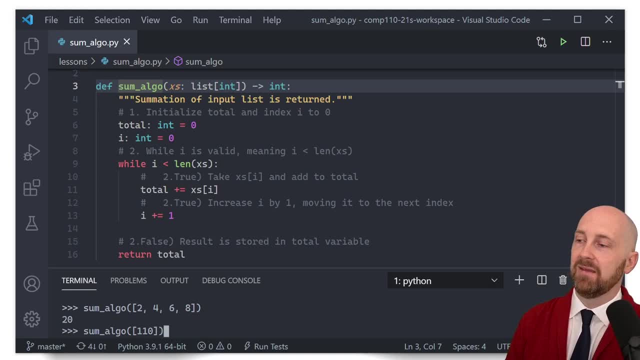 of, let's say, one item in our list, one ten, one ten. all right, so it seems like we've got, uh, the ability to have lists of arbitrary lengths, as our inputs here and our sum algorithm works, even though nothing changed about it. right, we didn't change any code. our algorithm is still the exact same. 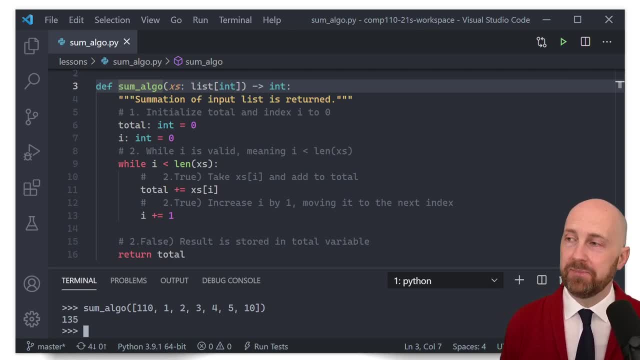 sequence of steps, but the way that we specified it in terms of a list and having each item in that list indexed and a loop which uses an index to move one by one through each item in our list, we're able to write this algorithm which abstracts this, these details, away from us. 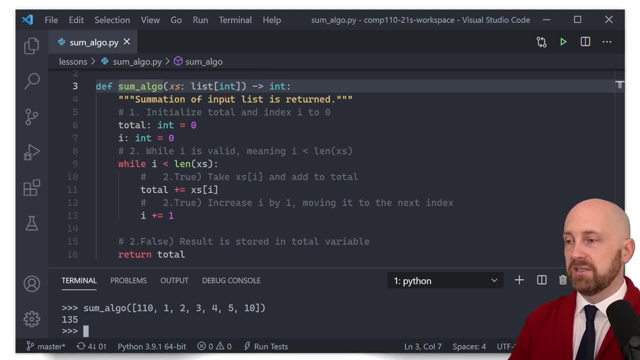 i should also mention that we don't have to use a list literal here. we could set up a list of, say, odds, right, which is a list of integers, and odds is going to be values such as, you know, one, three, five, seven. let's make the computer work a little bit harder here. we'll add nine to our list and uh. 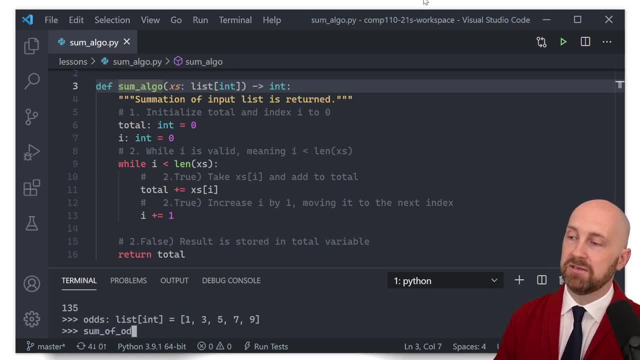 Now we could say sum of odds is an integer variable and we could store in that integer variable the result of calling sum algo with the odds input list, right. So because this is a function we can use as an argument that corresponds to the parameter x's. 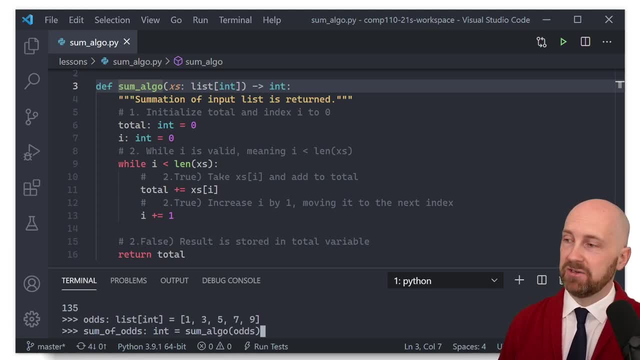 any list that's of the correct type, a list of integers, right, And it's going to return to us something of type integer, that the sum, and we're going to take that sum and store it in this variable right. So that statement has evaluated. 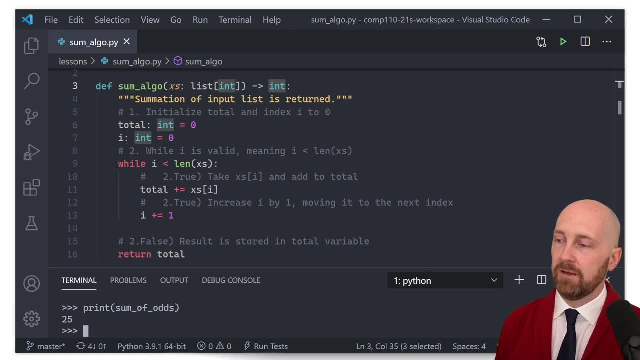 And so now, if we were to print sum of odds, boom 25,. right Now, I want to mention that when you're working in the REPL, you don't have to print your results, right? You can just access an expression and whatever if you write just a plain old expression. 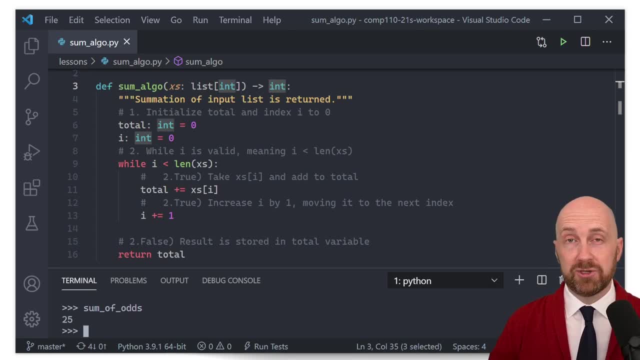 in your REPL. what REPL is short for is: read your input, evaluate it And then, if it's an expression, it's going to automatically print it for you. That's the P in REPL, And then the L is loop, And it's literally a loop. 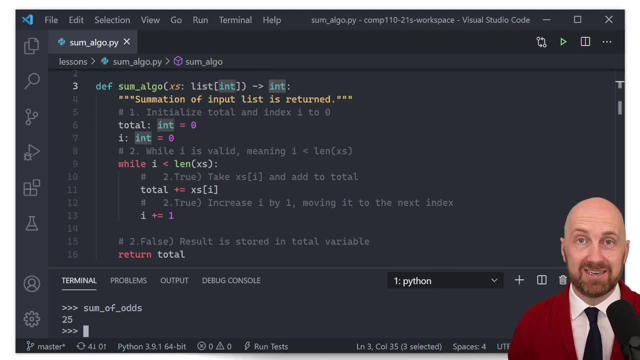 just like we're writing here. that brings you back up to the top and it reads your next line of code. It evaluates it, It prints the result. if it's an expression, Now it's different from you know. we had some statements here. 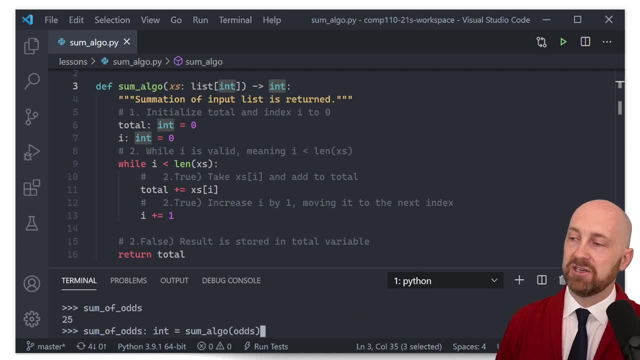 like you know, the statement here- sum of odds- is an integer that is assigned the result of the sum algo function being applied to the odd. So if we were to print the result, that's an odd argument. That's a statement. 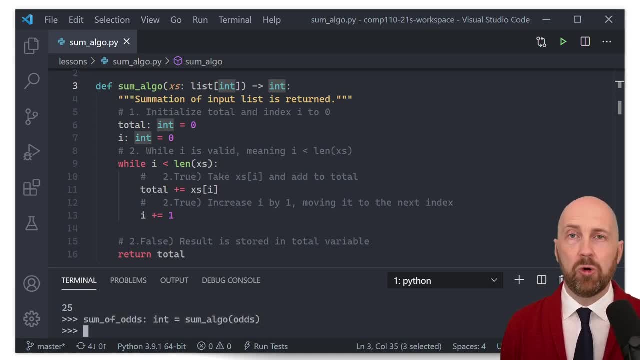 And because that's a statement, nothing gets printed, right? Only expressions when you're working in an, when you're working in the REPL will automatically get printed. This is different from when you're working in a stored program and you have to print something yourself, right? 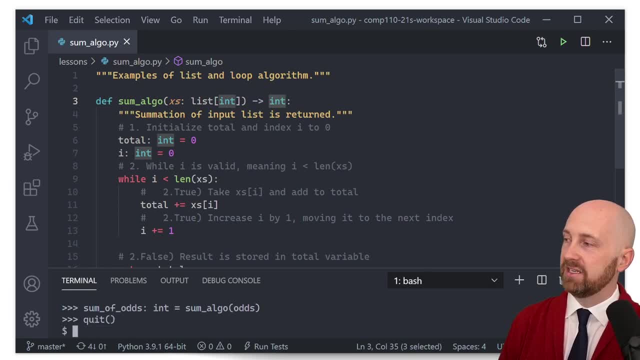 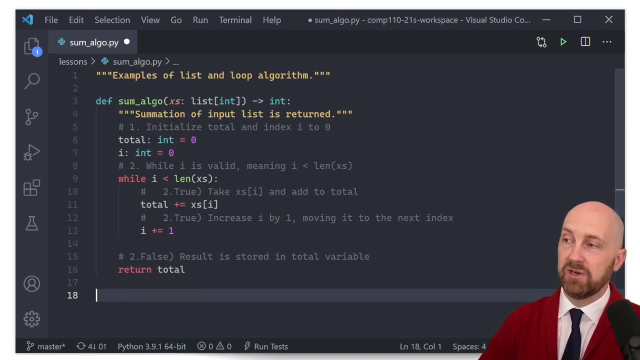 So just as one last example of that, if we wanted to add an example of calling this function to our program here I'm not going to go to the trouble of making a main function, but just so you have some notes and you can come back to this file. 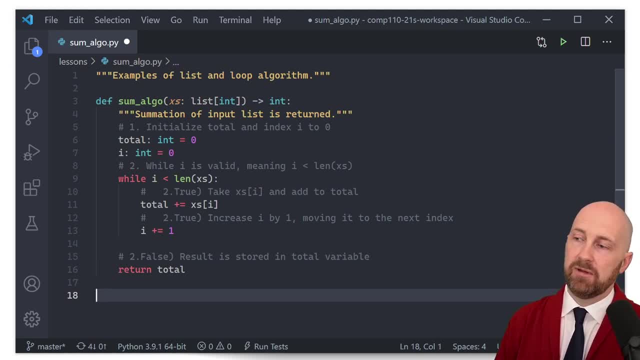 and understand how it's called. Let's try setting up a variable such as odds. That is a list of integers and that is assigned, you know, one, three, five, seven, And then we could do odd sum, which is an integer. 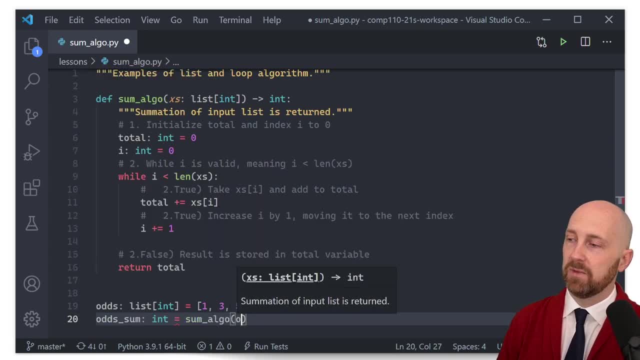 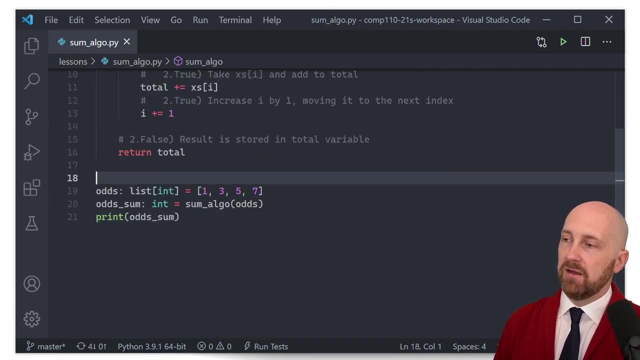 that is the result of calling the sum algo function with the odds list And then we can just print odds sum right, And we'll just make a note of this example usage. So let's say we're going to do odd sum algo function. 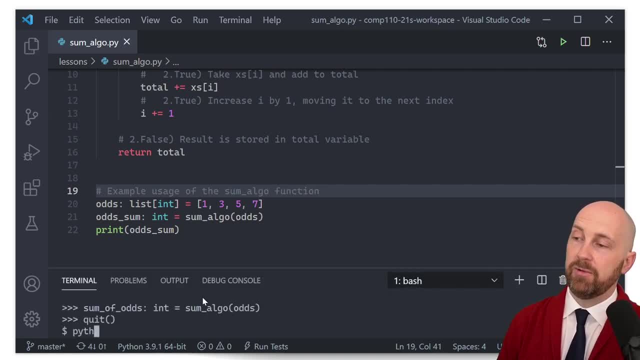 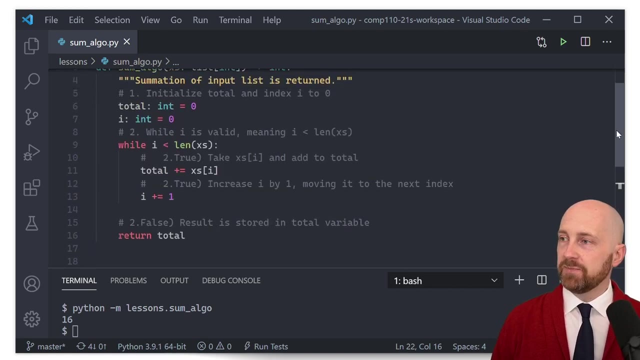 So let's say we're going to do odd sum algo function, All right. And now if I were to run this program, Python m sum lessons, dot sum algo, boom 16, right. So what we've seen in this video is the process of trying to describe an algorithm. 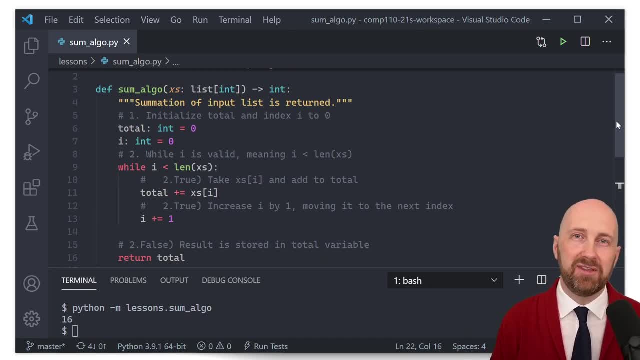 in English terms and in broad terms, and then think about: well, how can we bring this description a little bit closer and a little bit closer, Closer to a representation that we can write ourselves in a programming language such as Python, In this process of you know, 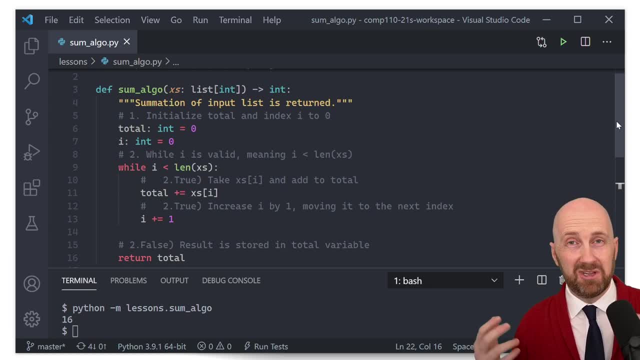 we'll start with some comments that we think of sort of as pseudo code, Like it's not really code. The computer has no idea what we're talking about, but we're thinking step-by-step in a way that we can then translate into Python instructions. 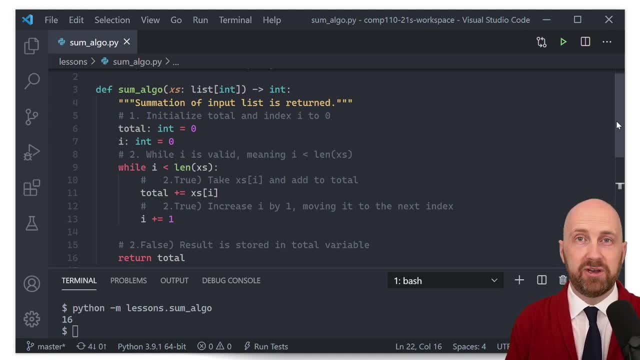 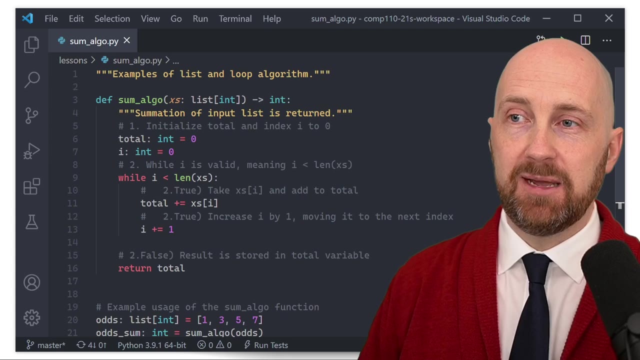 is a very common strategy for taking on new problems when you're trying to program and solve a new type of algorithm- And I do this all the time, even today. And what we've done, which is really neat, is we actually have our first example. 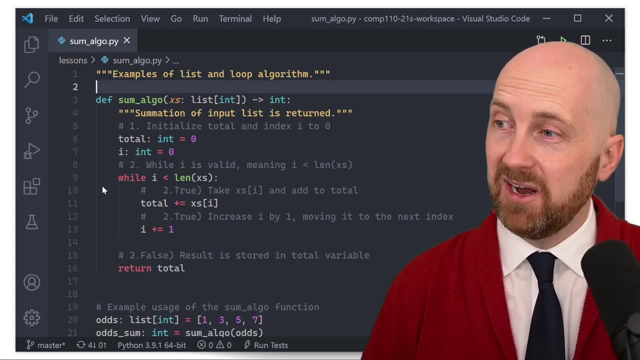 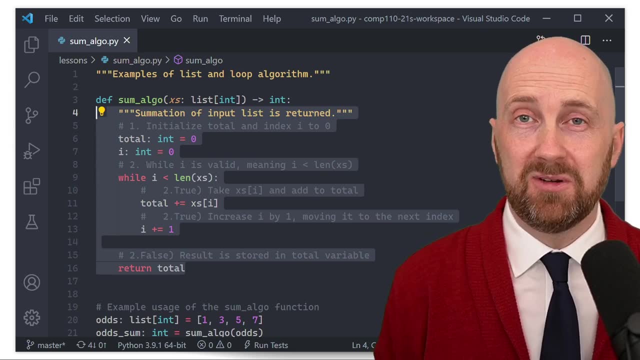 of a process abstraction. This is a process right, This idea of how do we take a list and from that list sum all of its elements and then return that result. That's a process that we had to think pretty deeply about in order to write this algorithm. 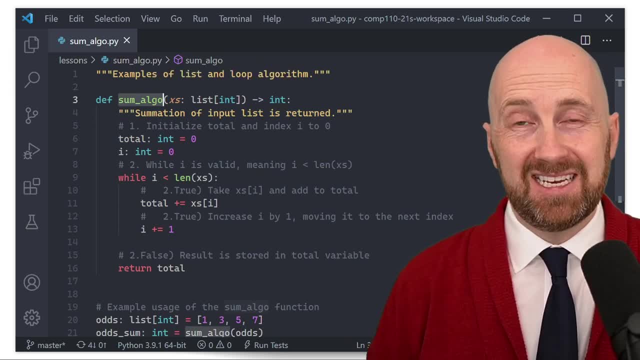 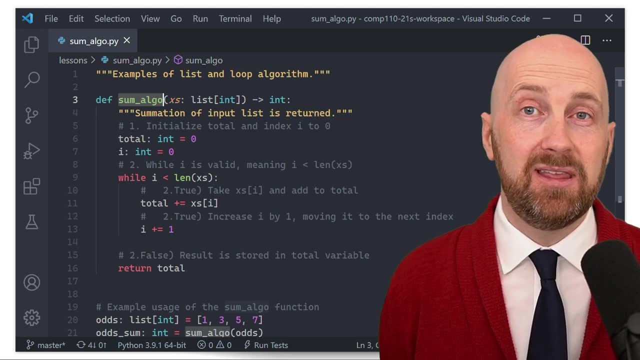 But once we've written this function, sum algo, that's an example of process abstraction. Now we can just use this function anywhere we want to carry out this task And we can think about it a little bit more, like we would think about it among ourselves as humans. 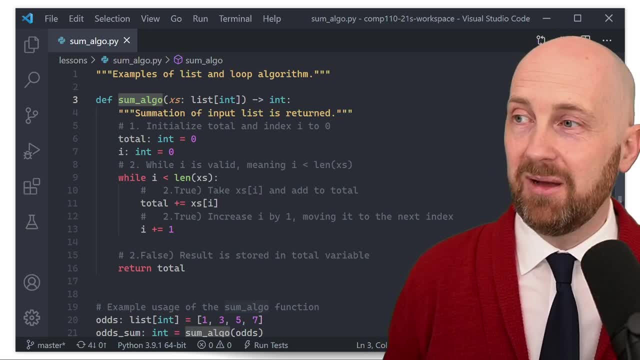 right, What do you want to? how do you add up a bunch of numbers? Well, you add them all up, or, once you've written this function, you just call the sum algo function and you don't worry about all those specific steps.